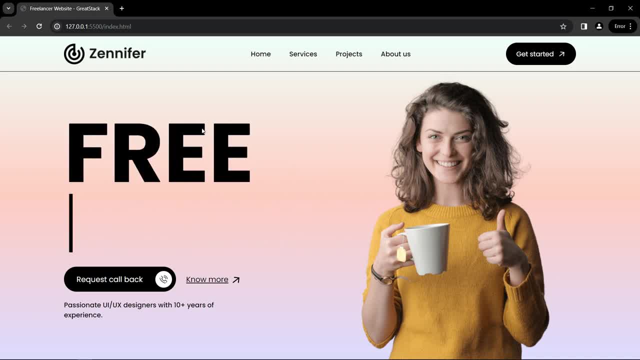 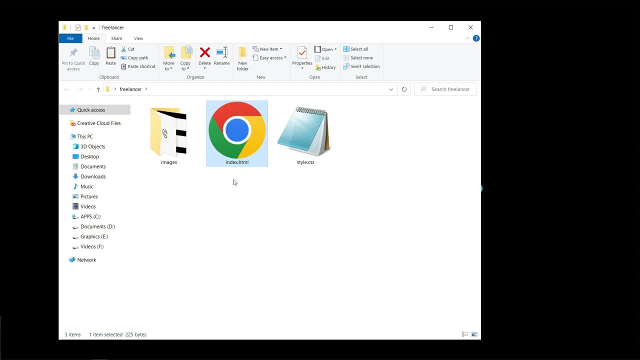 learn how to create a very simple javascript. So let's start this tutorial. Here we have this folder, and in this folder I have created one indexhtml file, stylecss file and one folder with some images and icons that I will be using on this web page. You. 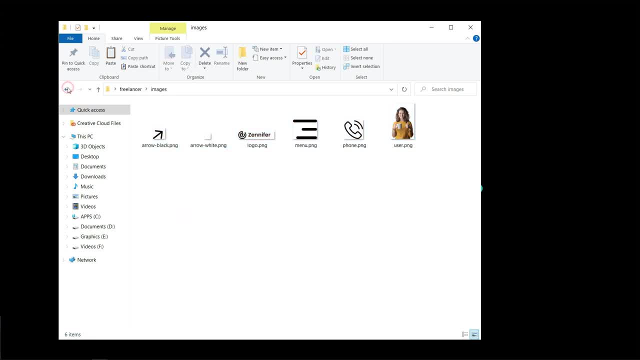 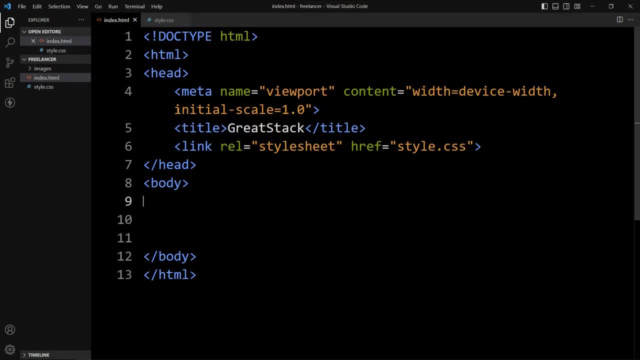 can find all these images download link in the video description. Now let's open these files with code editor, which is visual studio code. This is the indexhtml file where I have added the basic html structure. We have the meta tag, then title and link tag. 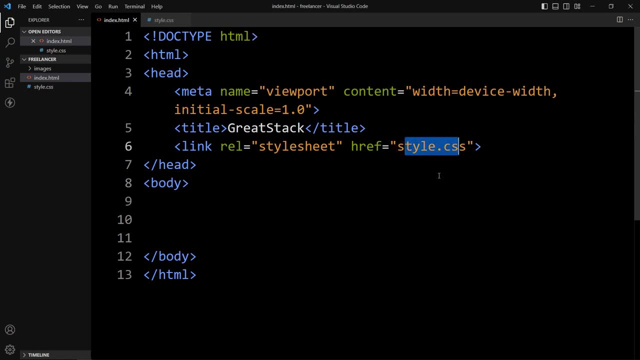 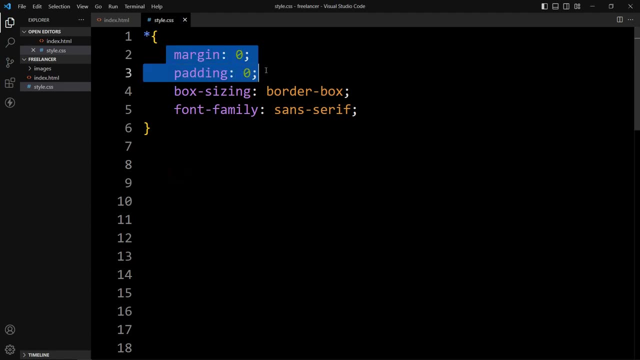 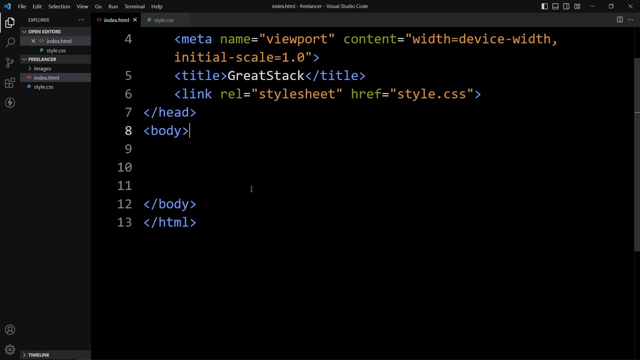 that will connect the html file with the stylecss file. So this is the stylecss file where I have added the global selector and added margin, padding, box sizing and font family. Now in this html file let's create some html tags. So first we will create the navigation. 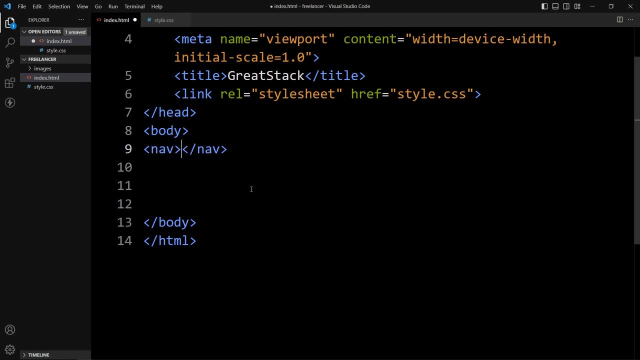 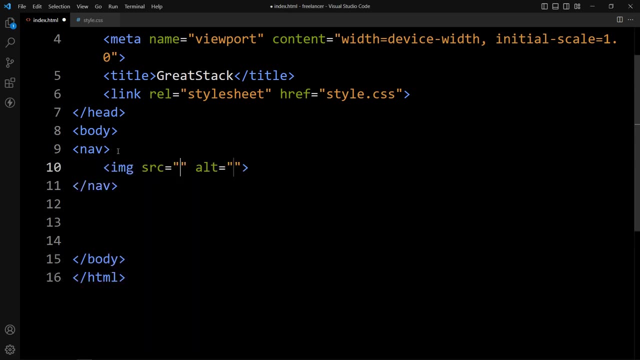 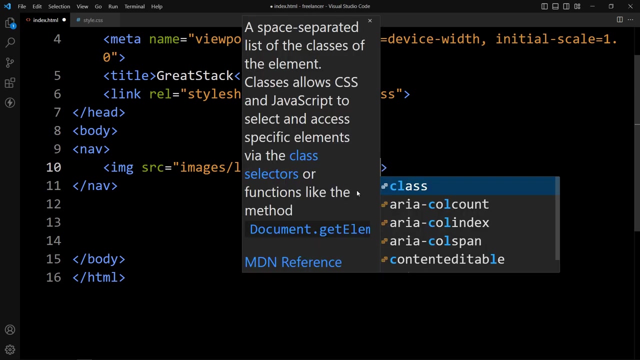 bar, so here i will use the nav tag. in this nav we will add one image that will be for logo, so let's add the file path images: slash logo dot png. this file is available in our images folder and here let's add a class name logo. after this logo we will add some menu links, so we will add. 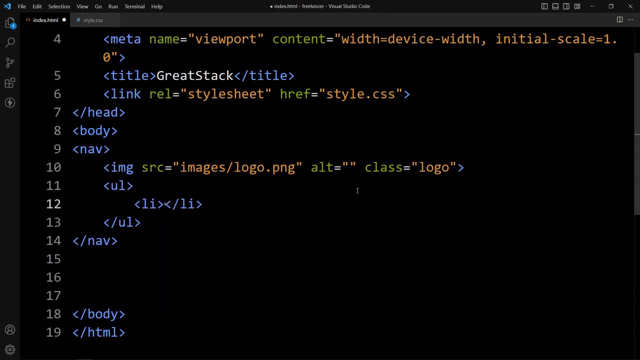 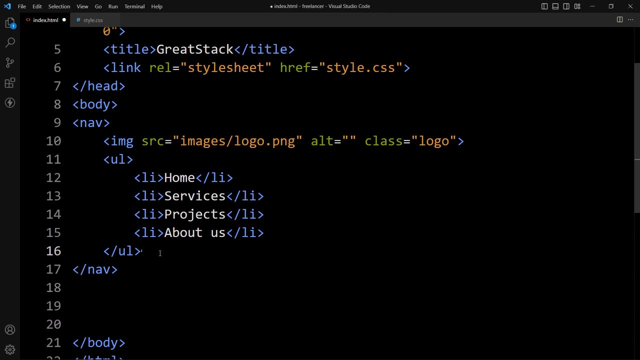 ul and li. so first menu link text will be home. now just duplicate it and we will change the name. after adding the menu list we will add one button. so here i'm adding the button and the button text will be get started, and in this button we will add a class name. 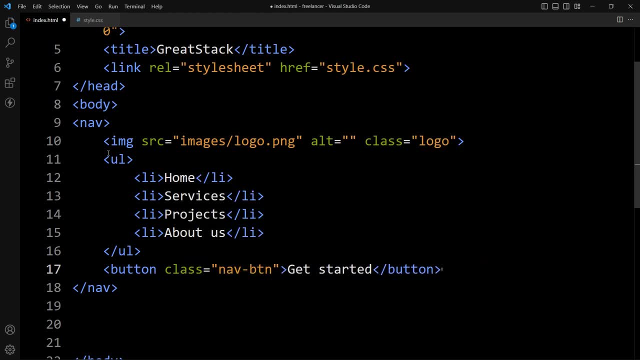 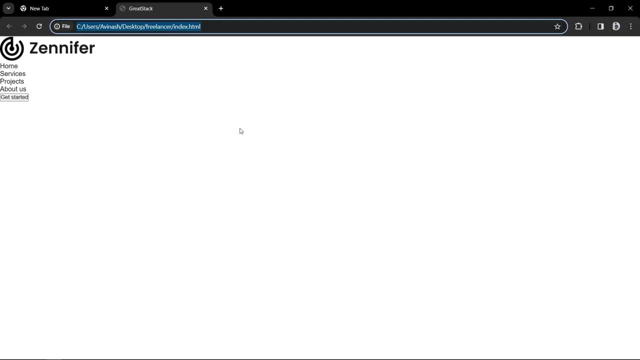 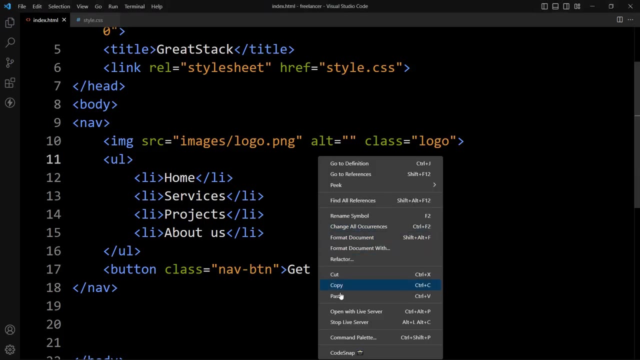 nav btn. so after adding this, let's open our html file. so come back to the folder and open this html file with any browser so you can see this web page. now we can open this web page with the live server. here we will select open with live server, so it will refresh the web page automatically. 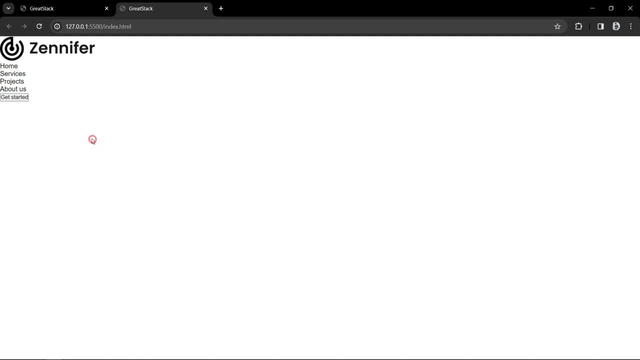 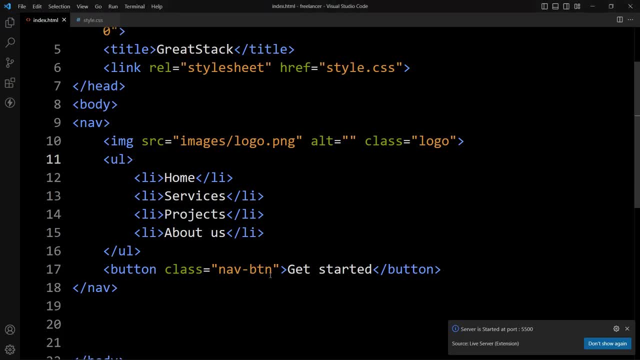 url has been updated, so we will add the same web page. but the url has been updated, so we will add let's come back and we will add one icon in this button. so here we will add one img tag and write the file path: images slash. this will be arrow, white dot png. after adding this, let's. 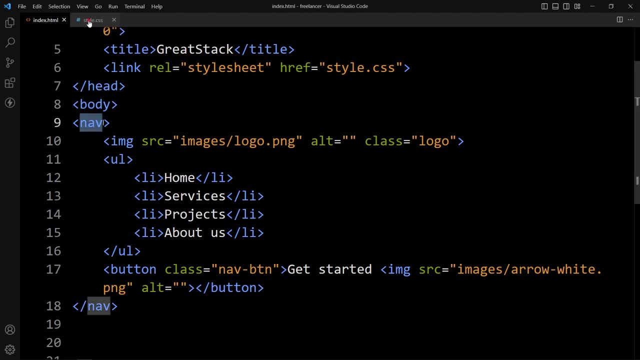 add this css. so here we will copy this nav and come to this css file. for this nav we will add the css properties. so for this css we will remove this setlem. now, if we do something in code我們 pour一 operators for this ng above css输入後 to this ne Chronicle tab whereby we Uhrent in kisser. 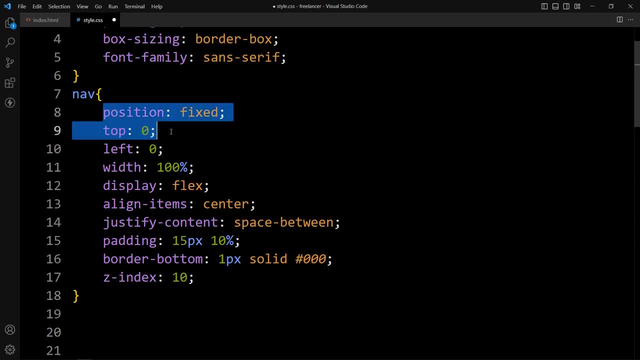 pentru ne diminuere the data to this quam matt. so for this cardです, We will add the css file for the. for this navigation bar i have added position fixed: top 0, left 0, so it will be fixed at the top whenever you will scroll the web page. we have added the width: 100% display flex. 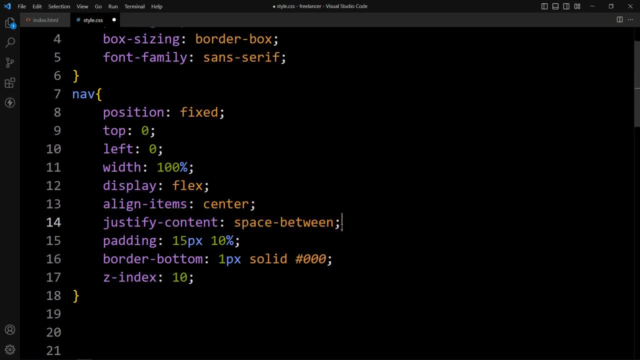 align item center and justify content space between. so it will align the contents side by side and there will be equal space between the logo, menu, links and button. then we have added the padding and border bottom, so there will be one line at the bottom of the navigation. 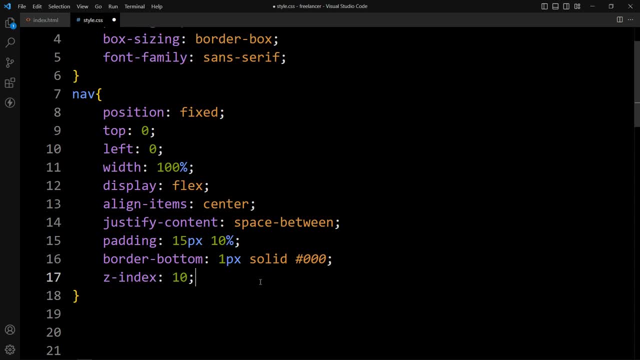 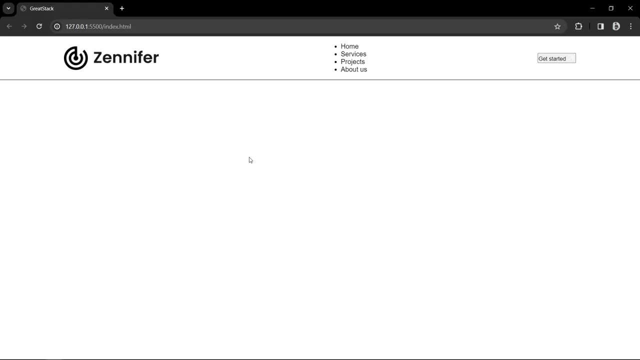 bar and z-dedex. so whenever you will scroll the web page, this menu will be always visible. after adding these css properties, let's come back to the web page and see the changes here. you can see we have the logo in the left side and button in the right side, and we have equal. 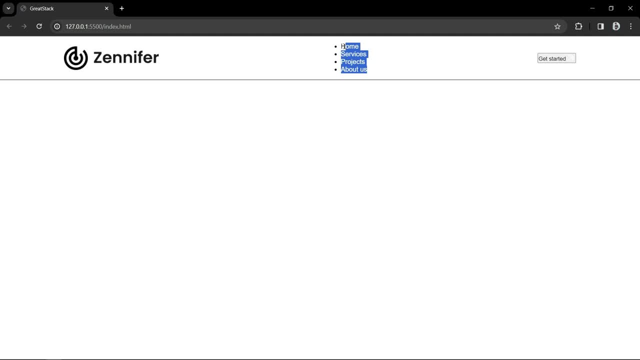 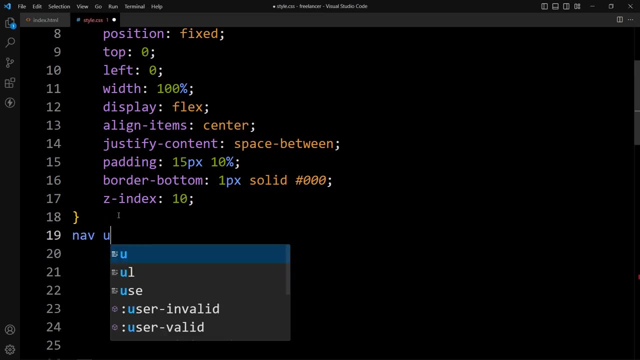 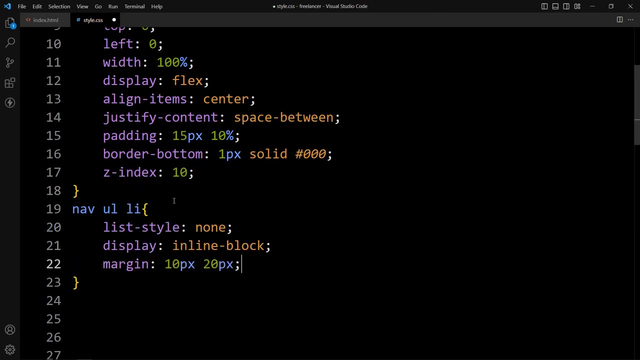 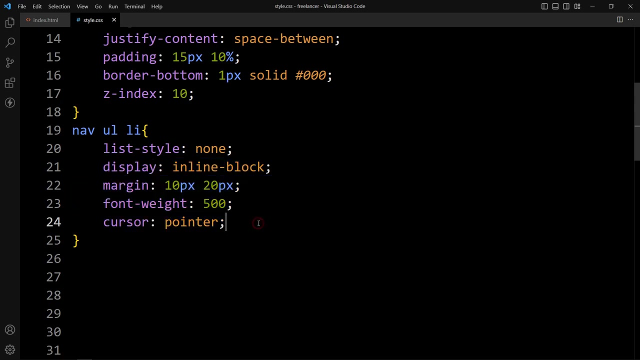 space here. now we have to align these lists horizontally and we will add some space also. so let's come back here. we will add nav, ul and li. so for this list let's add: the css is here. we have added lister style, display, margin, font, weight and cursor. 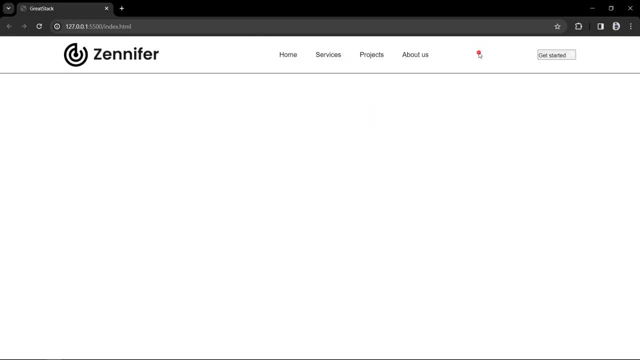 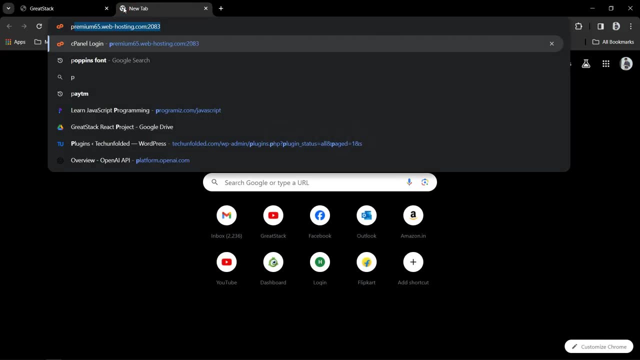 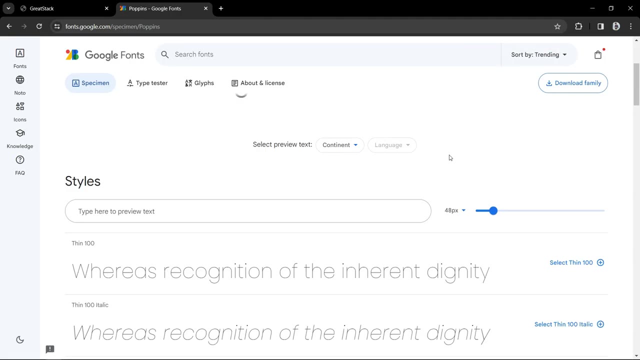 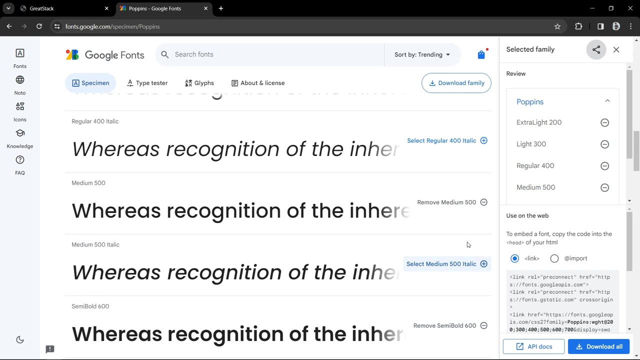 pointer, so you can see now it is aligned horizontally. next we have to change the font. for that, let's come to Google and search for poppins font. open this Google font website. from here you can select this: 200, 300, 400, 500, 600 and in the 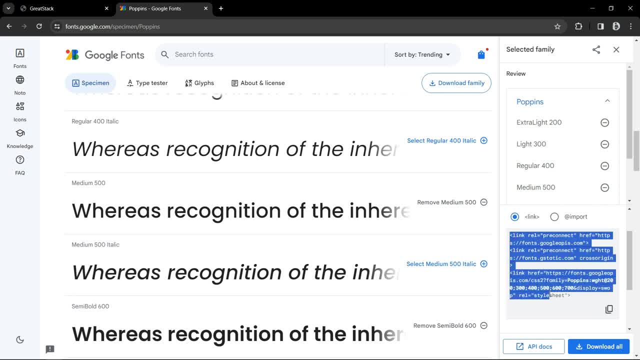 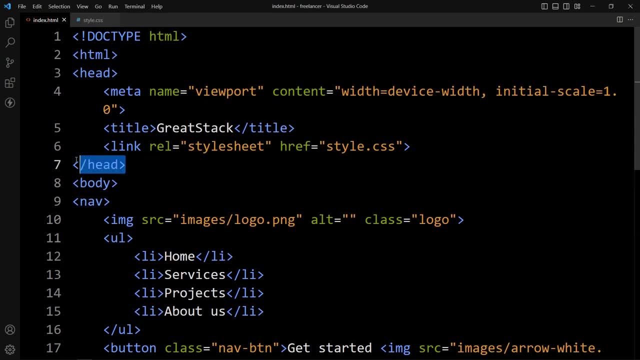 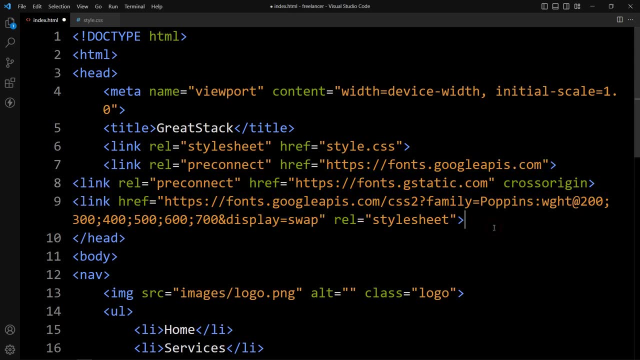 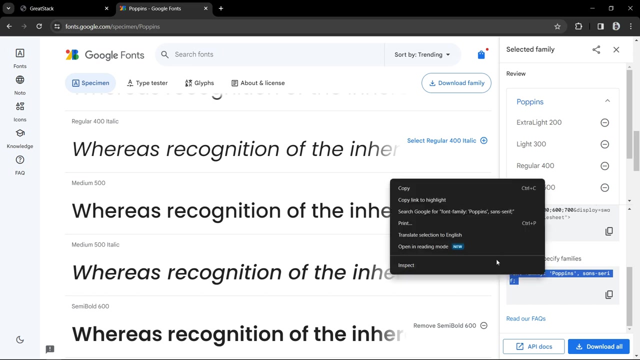 right side, you will get these links. so just copy these links and come back to the HTML file and place it here before this closing header tag. just place all these links. and now let's come back to the Google font website and here we have the CSS properties. just copy this one and come back to the CSS file. here we will place. 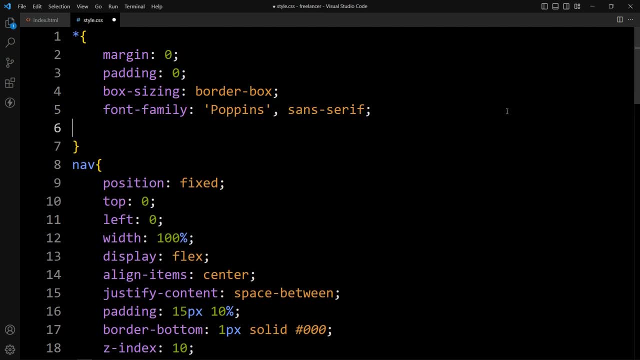 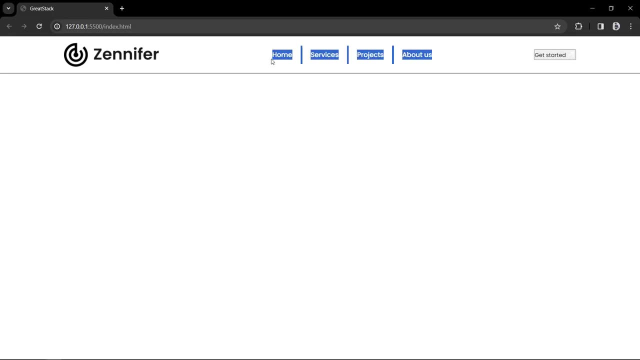 it at this line. font, family poppins and sensitive. after adding this, you can see the font has been updated here. after that we have to change the size of this logo. so let me come back and here we will add the CSS. so for this logo we will change. 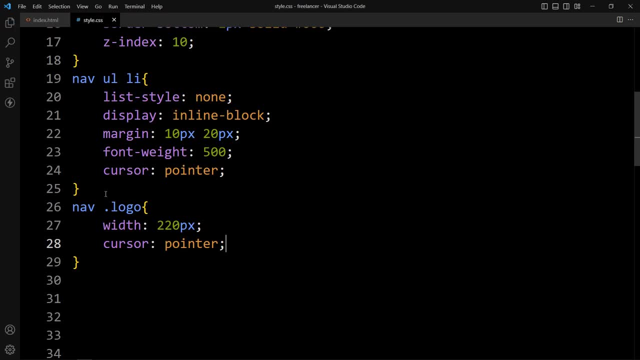 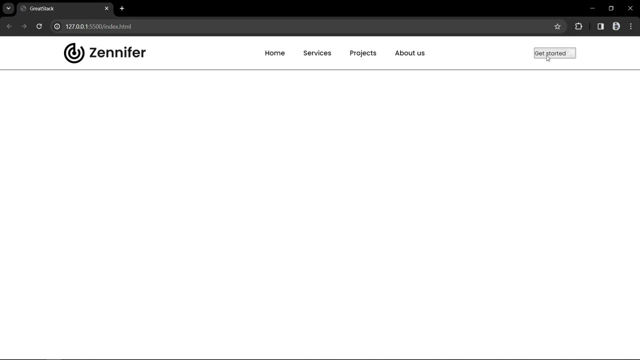 the width. after that you can see the size, for this logo looks perfect. next we will add the CSS for this button that is in the right side of the navigation bar. so let's come back to the HTML file and you can see we have the class name nav. 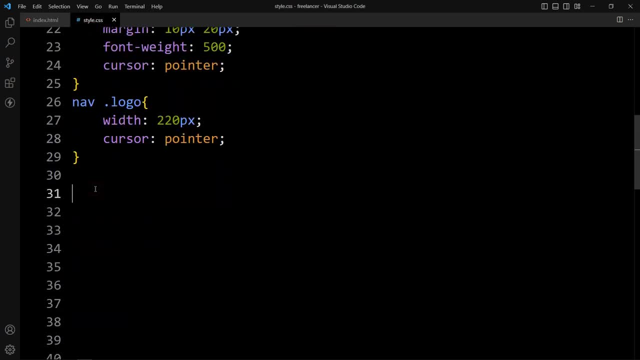 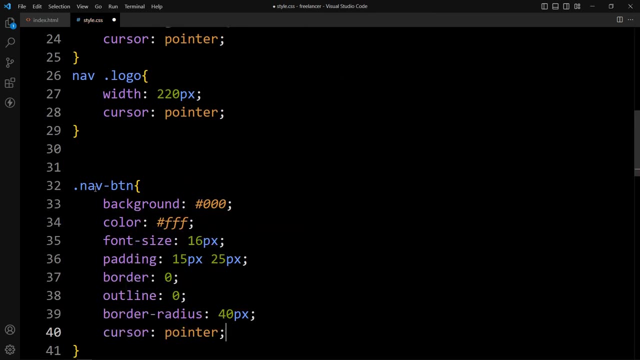 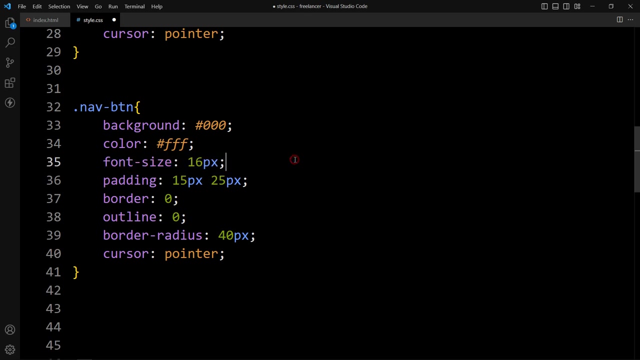 BTN. so we will add the CSS for this class name for this button. I have added the background, then color. this will be the font color. then we have added the font size and added padding. that will be space inside the button. then border zero, outline zero. then I have added the border radius of 40 pixels so that it will be round from the left. 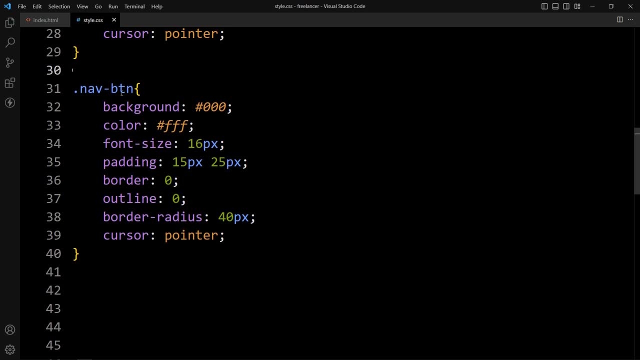 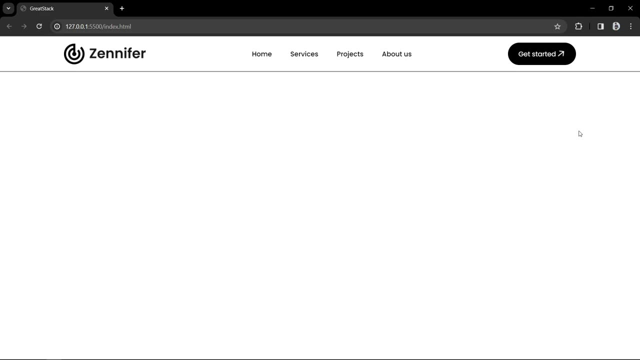 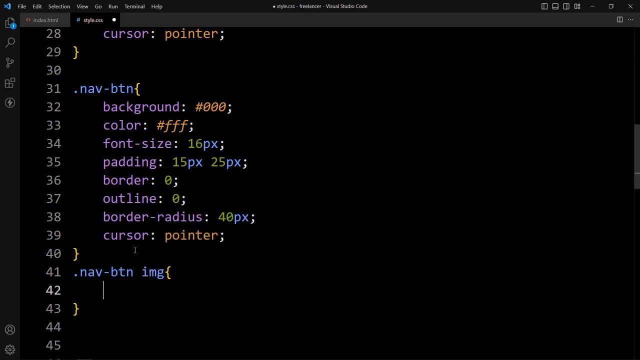 and right side. after adding this, you can see the changes on the button. now, in this button we have- let's change the size for this icon also, that is inserted using the IMG tag, so we will add the CSS for that image. so here we'll add IMG and for this one we 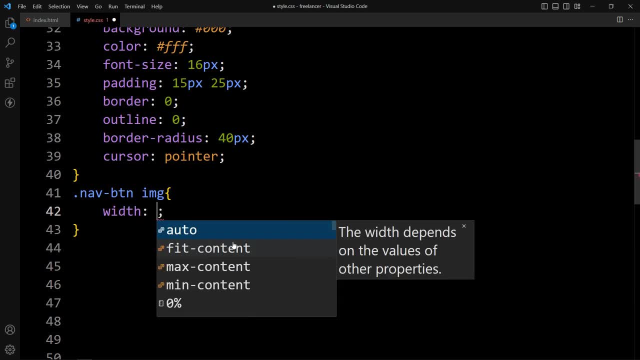 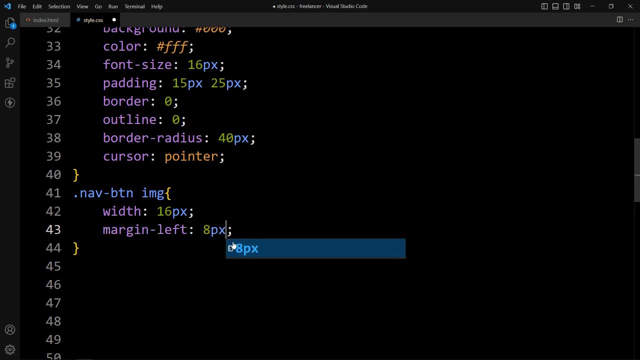 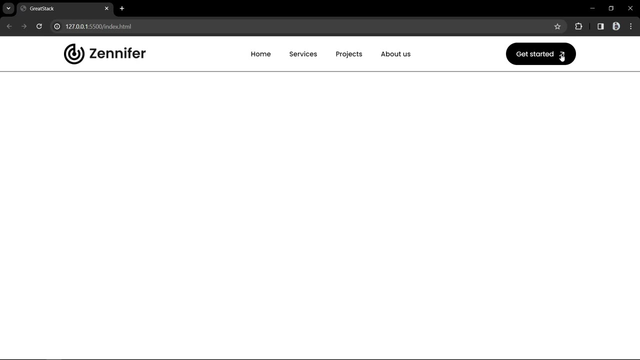 have to add the space from the left side and we have to change the width. after adding this, you can see the size, for this other icon looks perfect. now we design this navigation bar. next we have to create the other contents, like text and images. so let's. 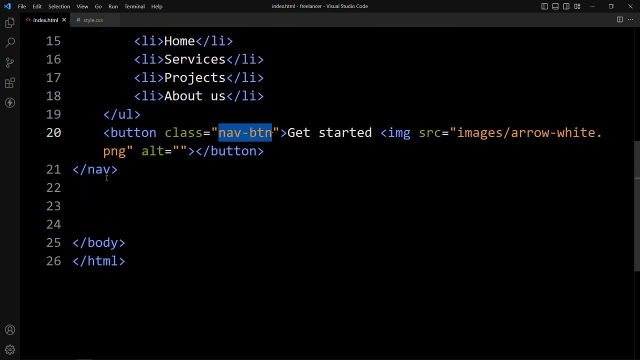 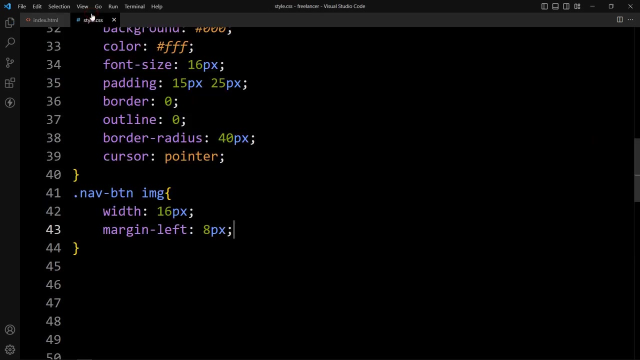 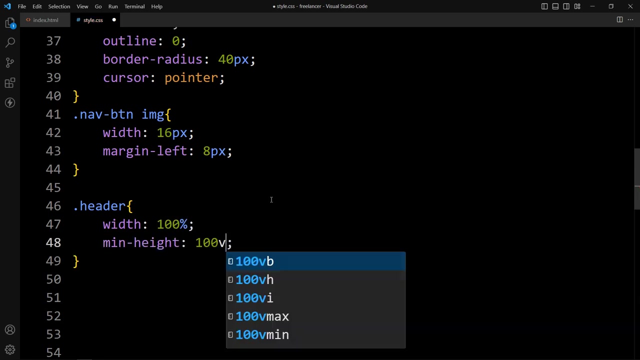 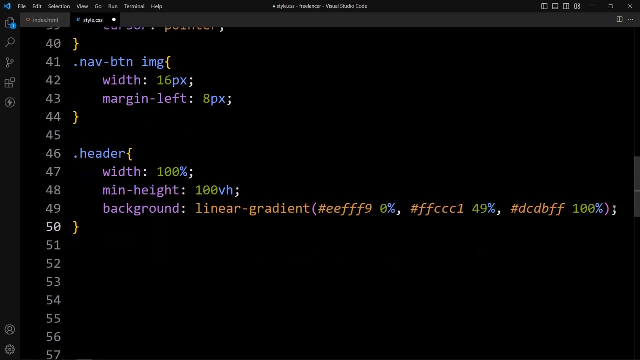 come back to the html file and here, after this closing nav tag, we will create one div with the class name header. so let's add the css for this header. just copy this, add it here. now for this header we will add the css properties. so for this header i have added the width and minimum height. then i have added canvass test, for which let me add some volume and let's skip this one for every one. so during the slow class i have added the Nigeria sort list, for which i happened to stop the sour года for the second time and i thought i just said the same thing from the second time. i 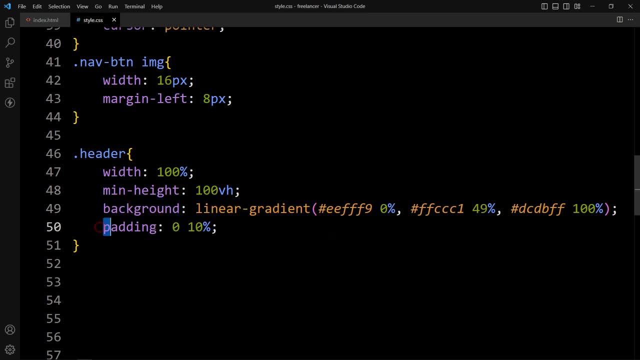 updated the questioning window, which is are tractor search here at large fox. so i also added the first column of to add the class name header like this. so go back to the. Så we have noodles a little, the linear gradient color in the background and padding. that will be 10%. 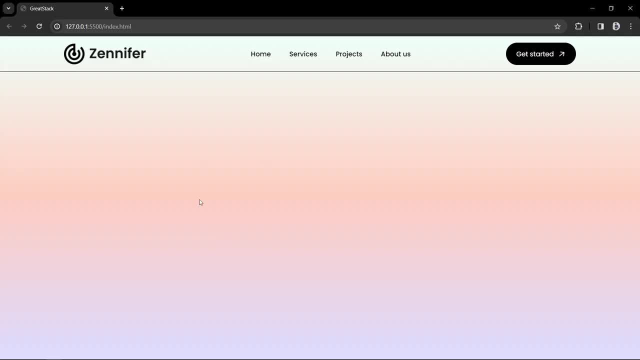 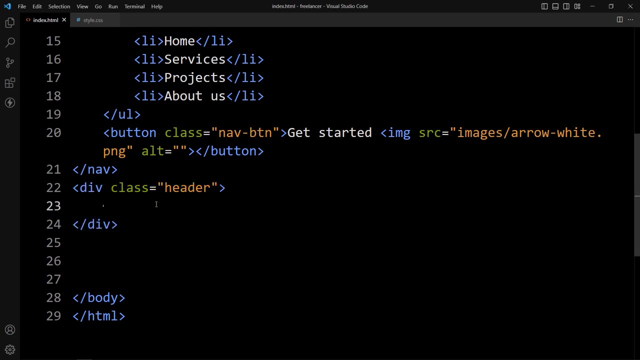 from left and right side. so after adding this, you can see we have the gradient color on this complete web page. now we will add the text and buttons. so let's come back to the HTML file and within this header let's create one title in the h1 tag. so here we'll add h1 and here we will add the text free and will. 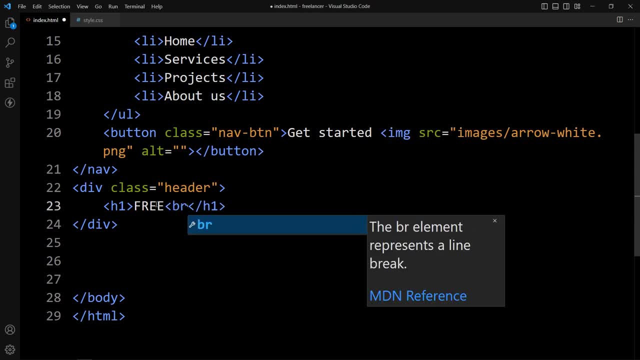 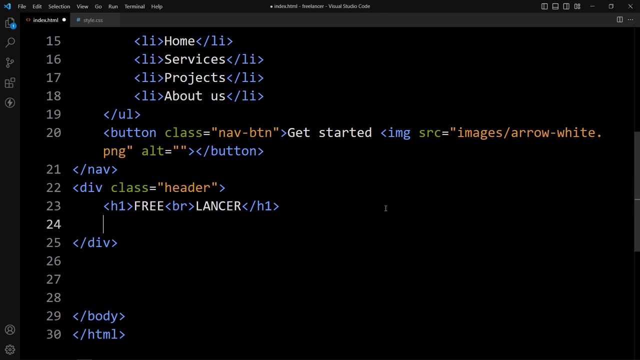 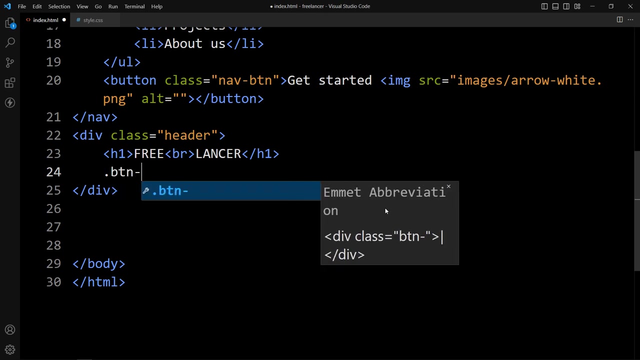 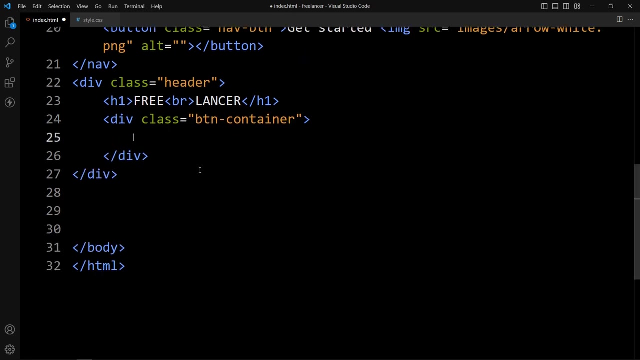 add the line break. freelancer, we have the line break here. after adding this title, we will add one div that will contain two buttons. so we will add one div with the class name btn container. in this btn container we will add buttons, so let's add the button tag and here we will add the text. 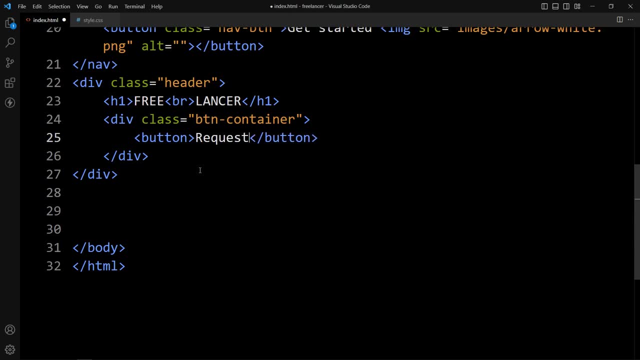 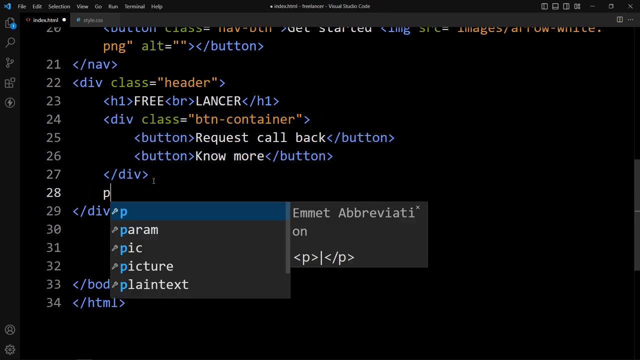 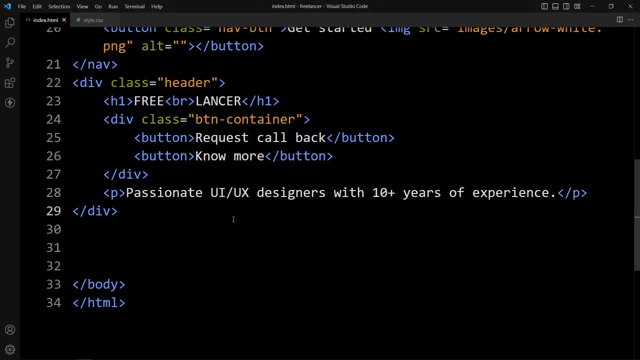 request callback, and there will be one more button, or you can say link. it is no more, and after that here we will add one text in p tag. so this is the text. after adding this, let's come back to the web page again so you can see. the title is behind this. 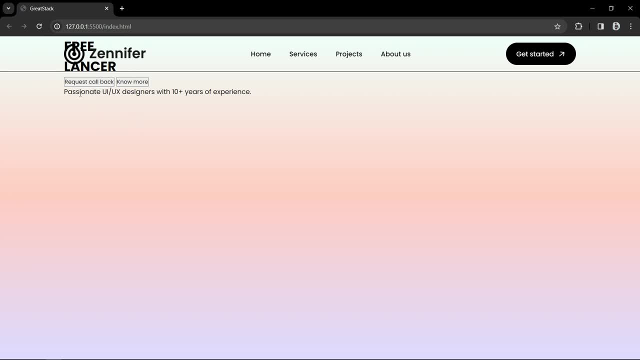 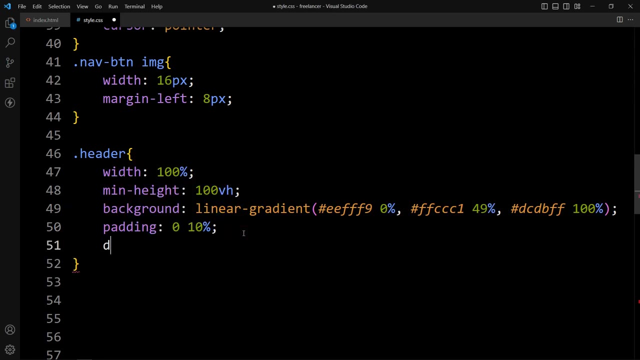 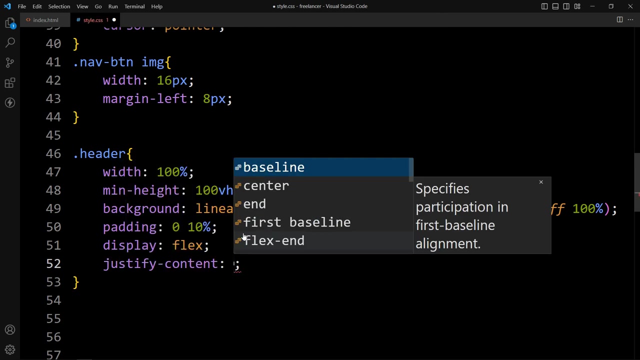 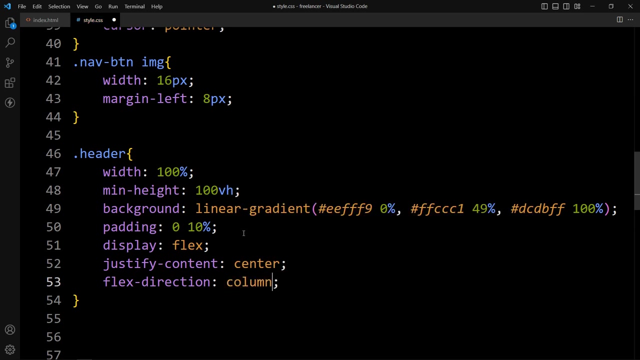 logo. so we have to change the position and we have the buttons here and this text. so let's add some css properties. so let's come back to the css file and in this header we will add display flex, let's content center and we will add the flex direction column so that all the 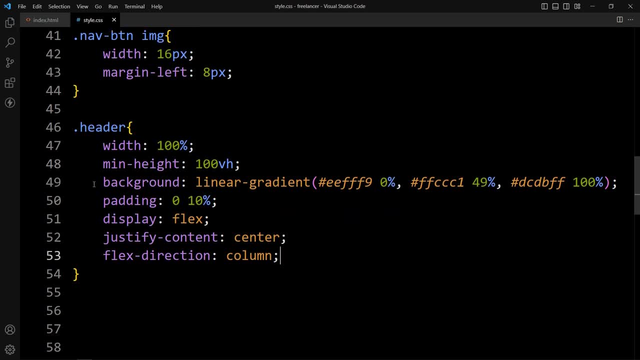 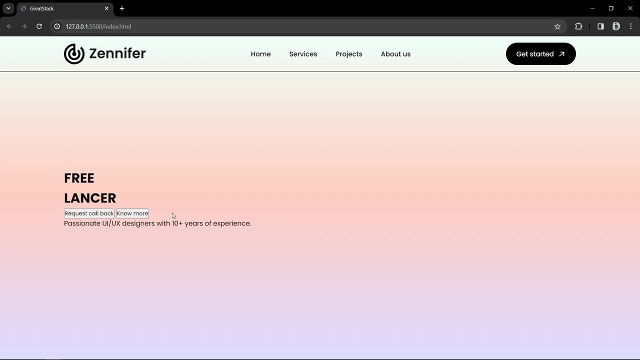 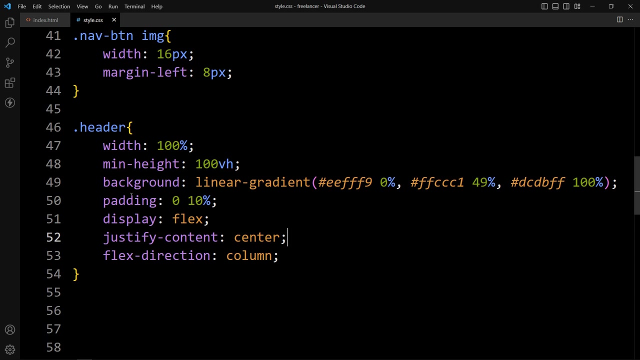 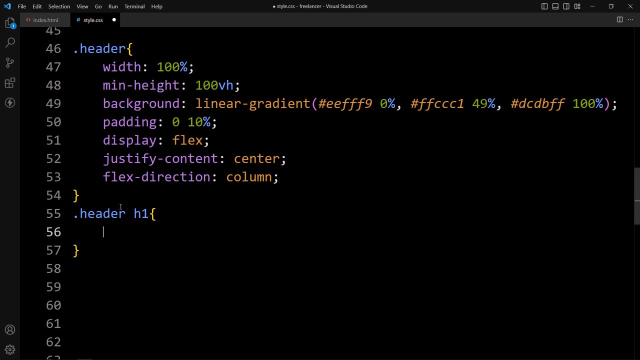 text will be vertically centered. so after adding this, you can see these contents are vertically centered. now we have to increase the font size of this text and we will add the line height. so let's come back and here we will add header h1. for this h1, we will add the margin from the top to add some space. 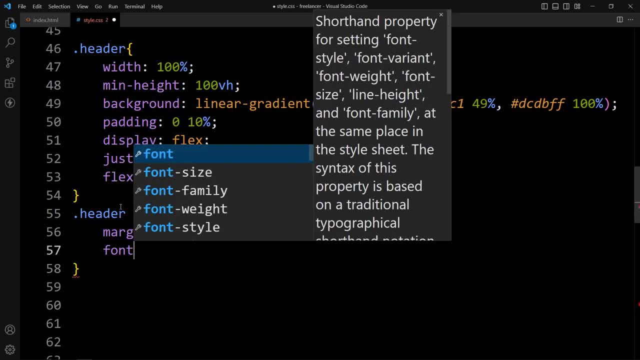 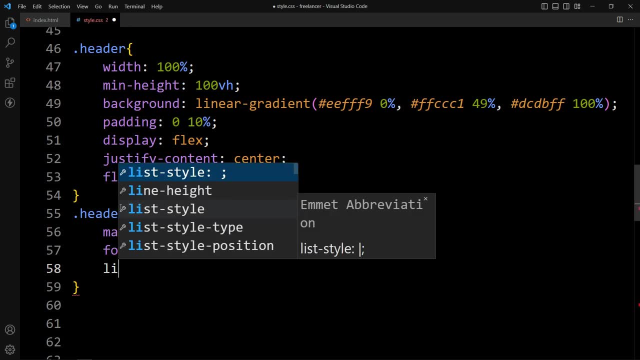 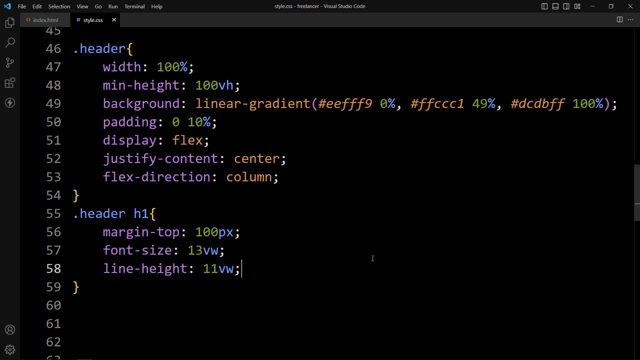 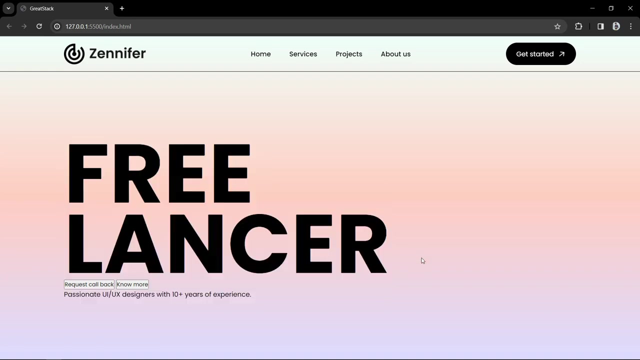 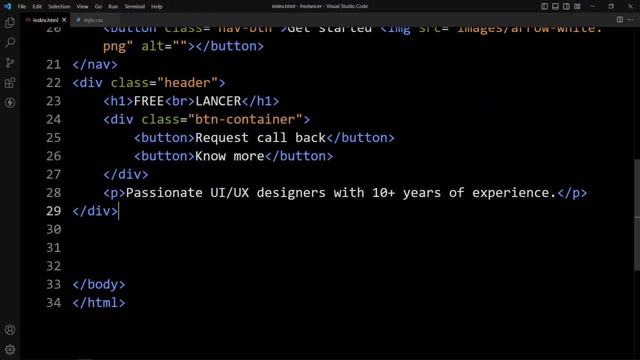 and font size will be 13 viewport width. then line height will be 11 viewport width. after adding this, you can see the font size and line height for this text is looking perfect. next we will add the space above this button. so here we have the class name. let's copy this btn container class name, add it here. here we. 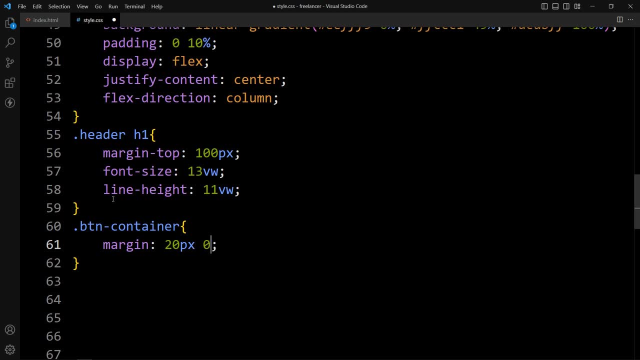 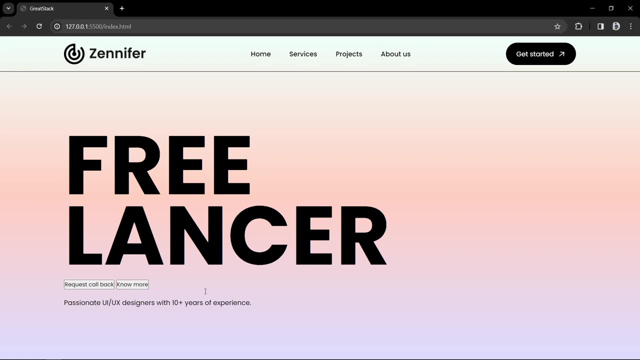 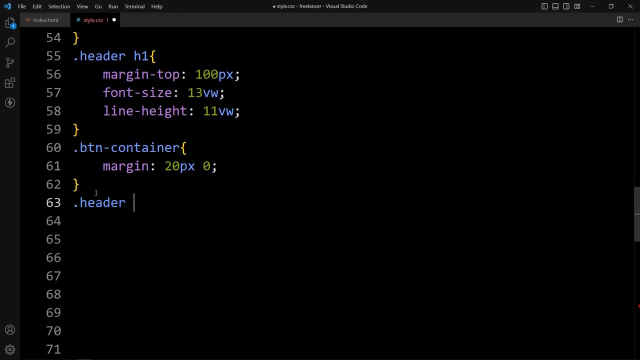 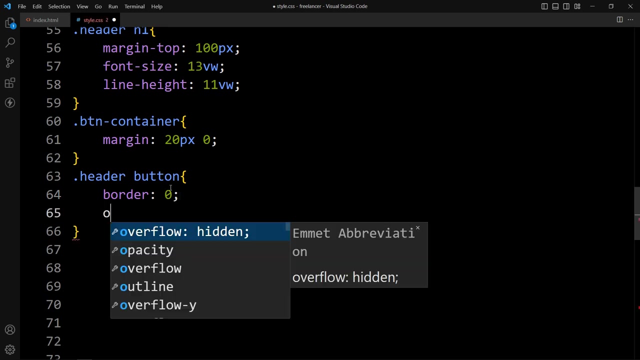 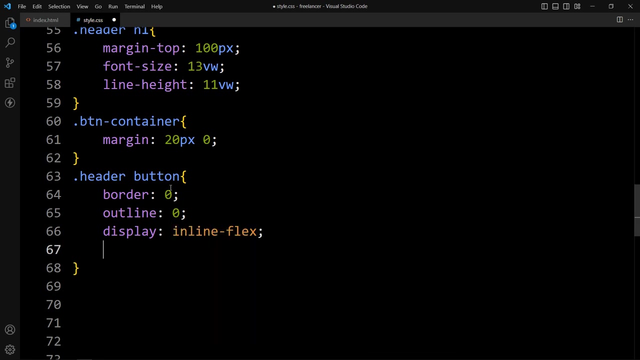 will add the margin of 20 pixel from top and bottom, left, right, 0. now we have some space around this button. next we have to design this button, so here we will add dot header and button for this button. we will add border 0. then outline 0. display will be inline, flex align items: center. font size will be 18. 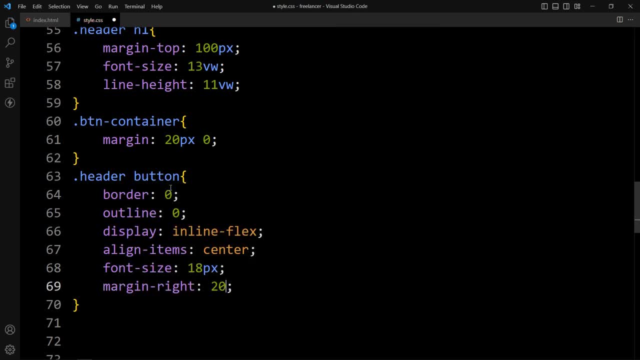 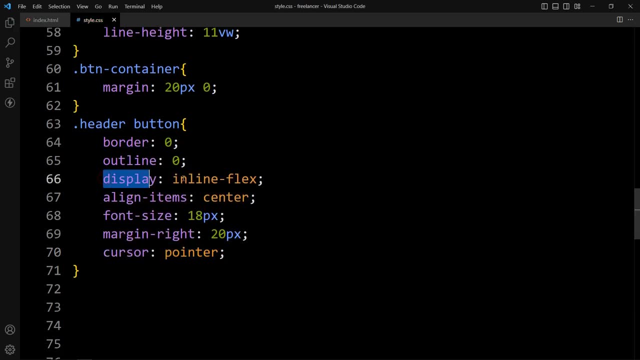 pixel and margin right: 20 pixels, so that we will get a space between both buttons and cursor pointer. here we have added display inline flex align item center, because in this button we will place the icons also, so that the text and icons will be aligned horizontally. here you can see we have 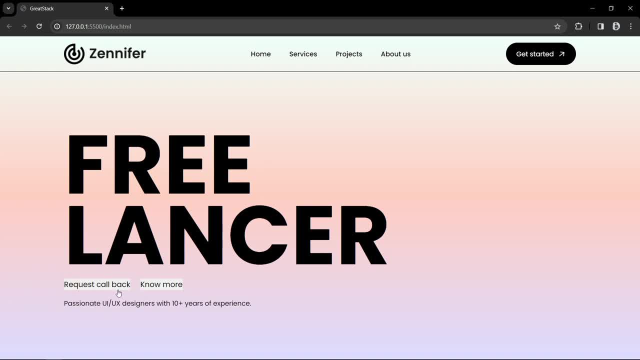 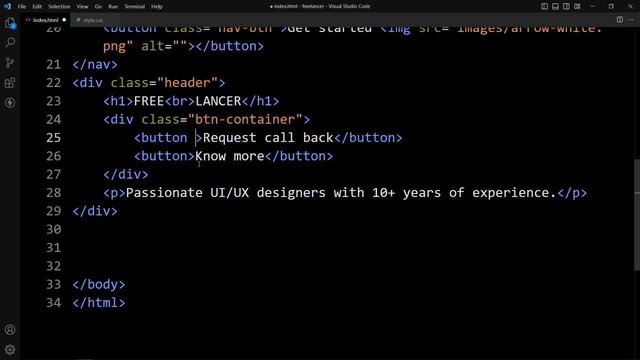 only text. so we will add the icons also. now we need different background color in the first button and in the second button. the background for the second button will be transparent. we will add the different Mc beat class name. so here we have two buttons like. so in the first one let's add the class VTn- dark sign. 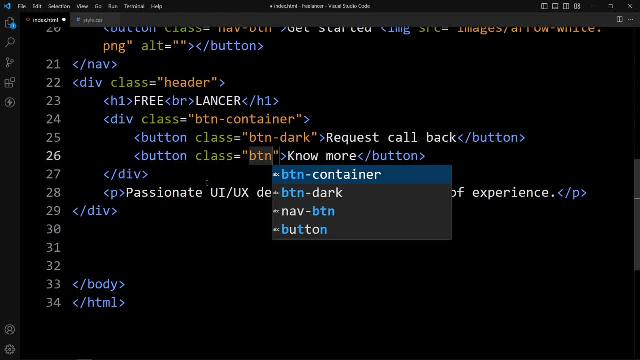 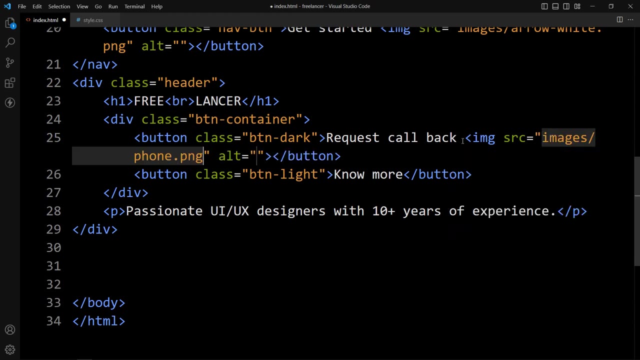 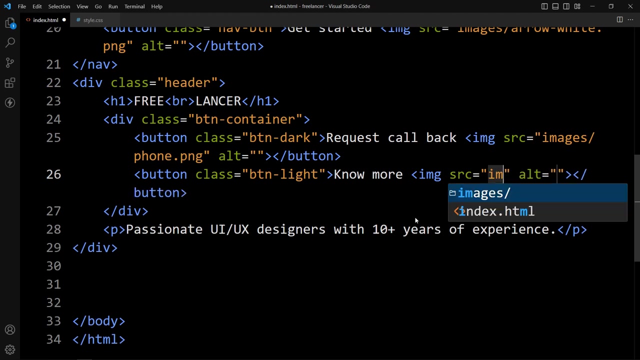 in the second one we will add the class name VTn light. so our emoji icon goes like this: so the next button isvuoro Vvo grande. the file path images: slash phone dot png. and here in this second button, after this text, we will add the img tag: write the file path images: slash arrow black dot png. so we have. 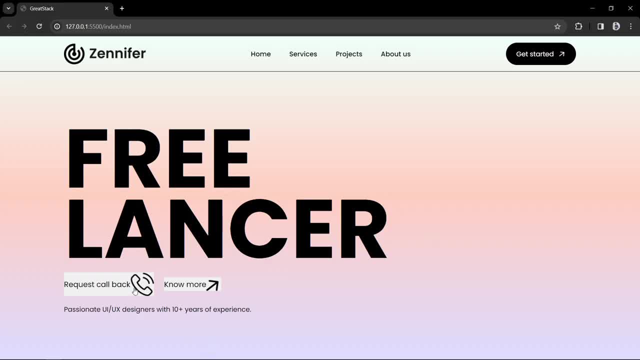 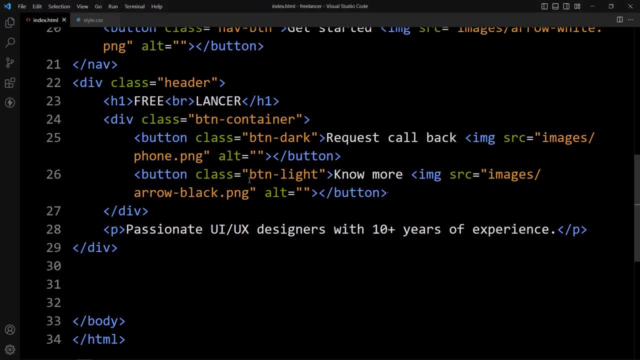 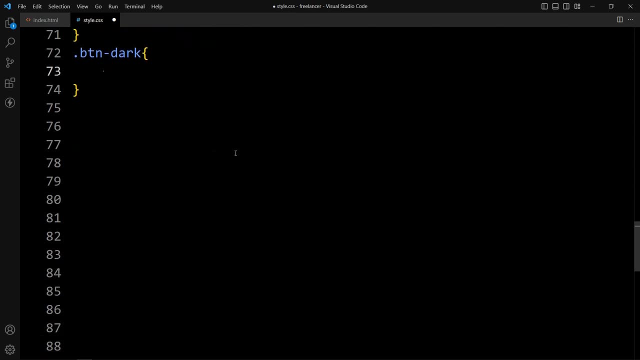 added two icons. you can see we have these icons here now. we will add the css properties for the dark button. so let's copy this class name btn dark, place it here in this css file. so for this button, let's add the css properties in this button. we have added the background. 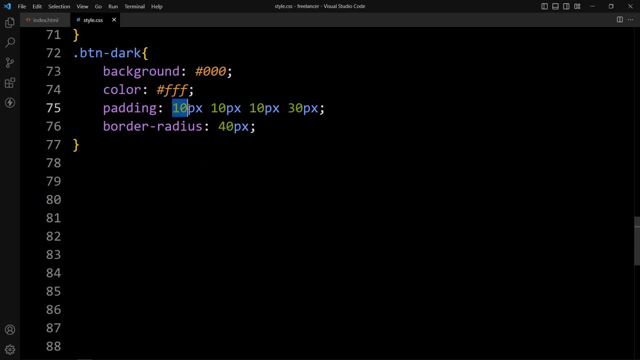 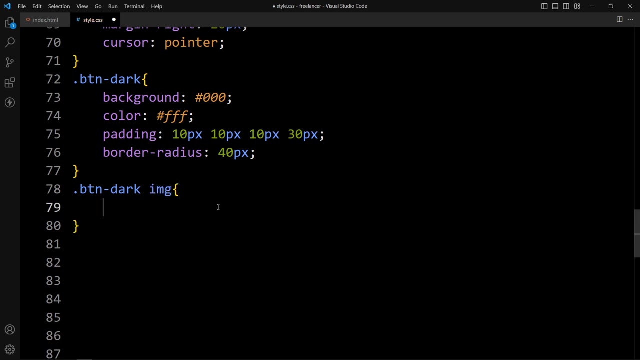 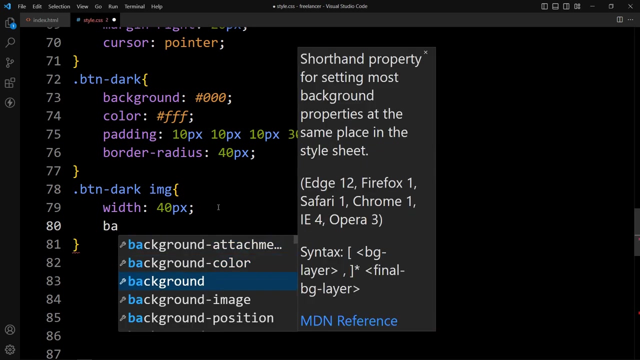 and color. then we have added the padding. this is from top, right, bottom and left. in the left side we have added 30 pixel, then border radius of 40 pixel. in this one we have the icon also, so let's add the class name, then img. in this one let's add the width, the background. 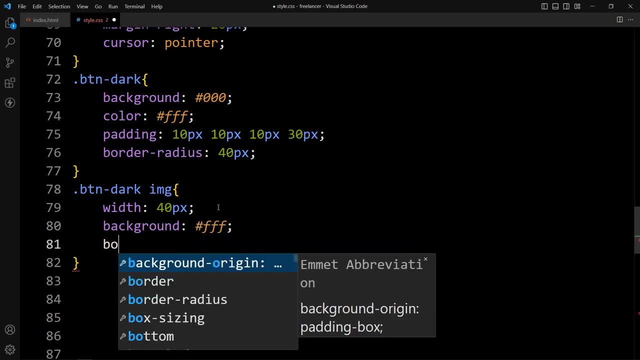 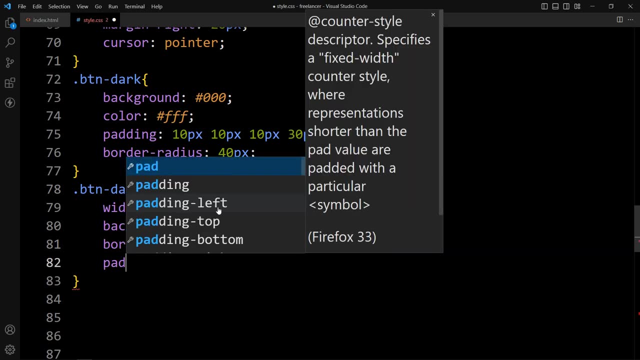 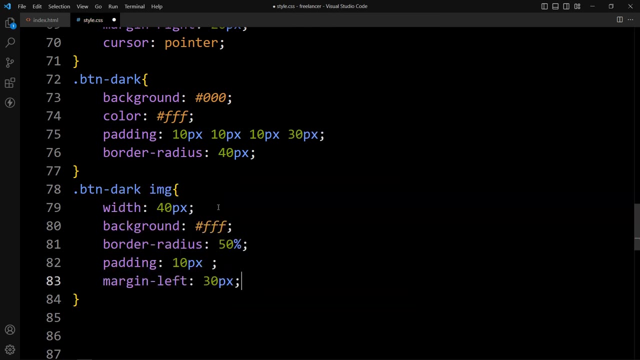 will be white for the icon. border radius 50%, so it will look like a circle. then you will add the padding of 10 pixel and continuously add the background to it. after that your course is ready. margin left: 30px. after adding this, you can see the first button looks good. next we have 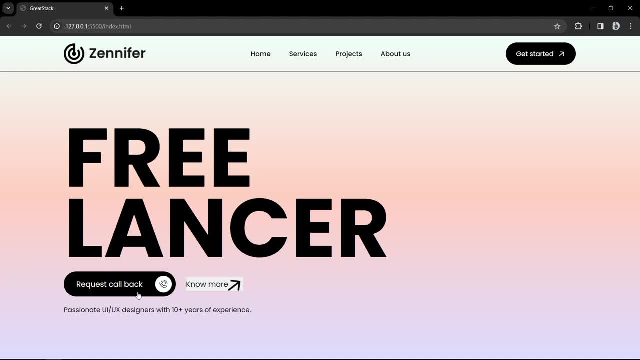 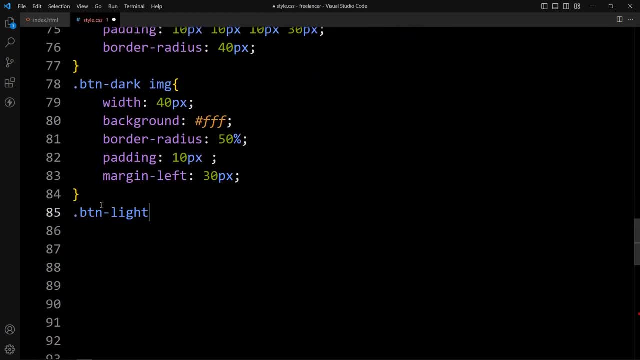 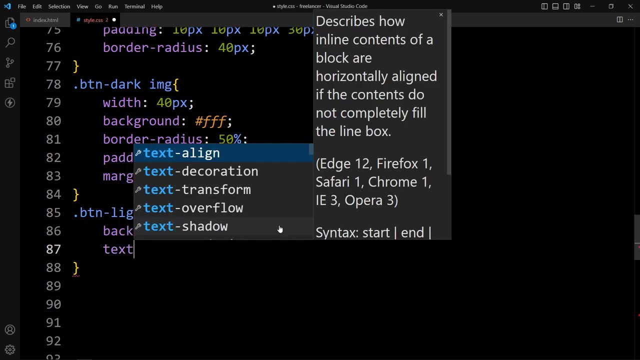 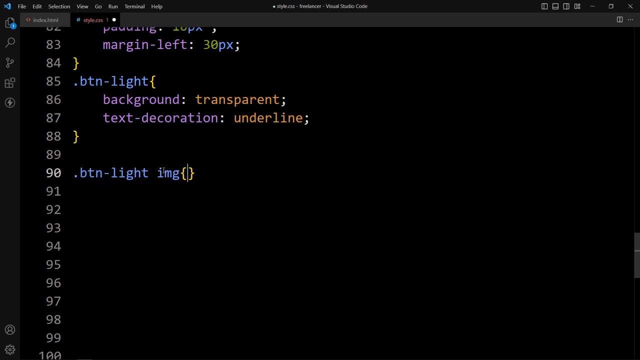 to add the css for the second button, which is btn light. so just copy this class name btn light, add it here, and here we will add background. transparent text decoration will be underline and in this one we have the icon. so we will add the img tag and for this image, 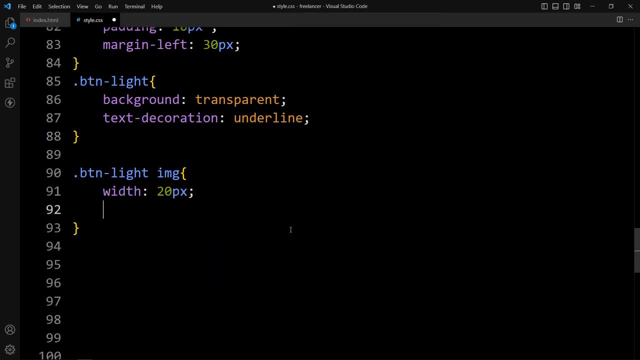 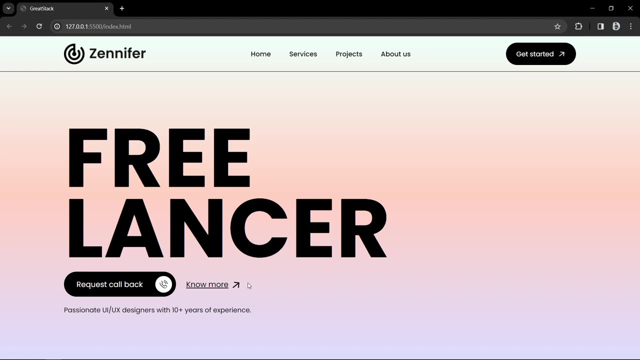 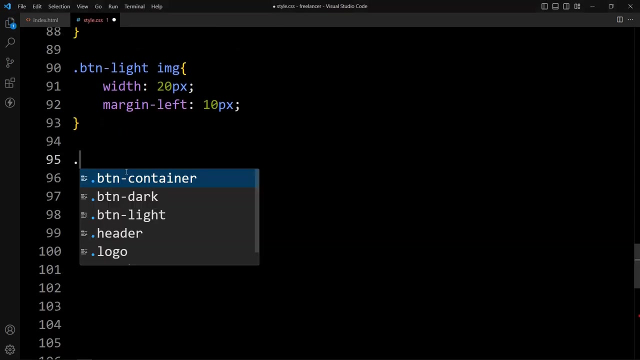 the width will be 20px and space from the left side, so margin left 10px. so this- no more link is looking good. next we will add the css for this paragraph text. so here let's add header and p. so for this. 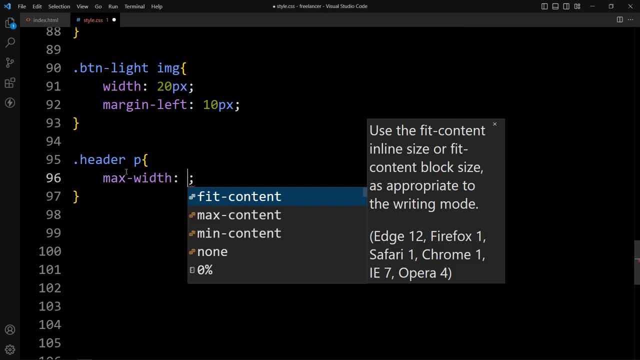 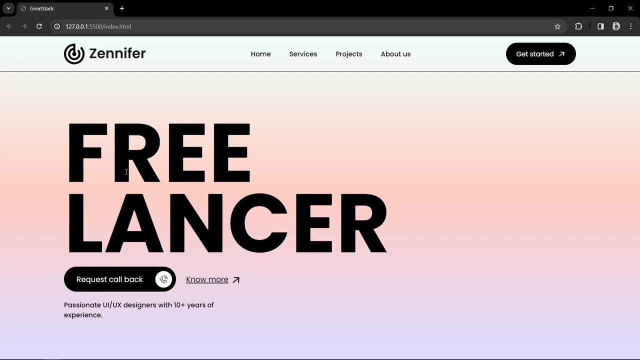 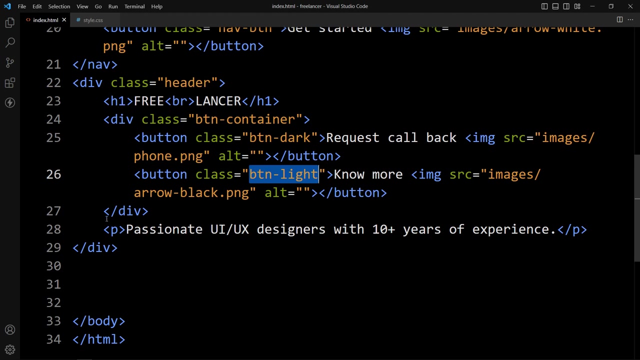 p tag. we will add the maximum width. it will be 360px, and font weight will be 500. now this text looks good. after adding this, we will add one image on this web page to place the image. let's come back to the html file and after this p, here we have the p tag. so here: 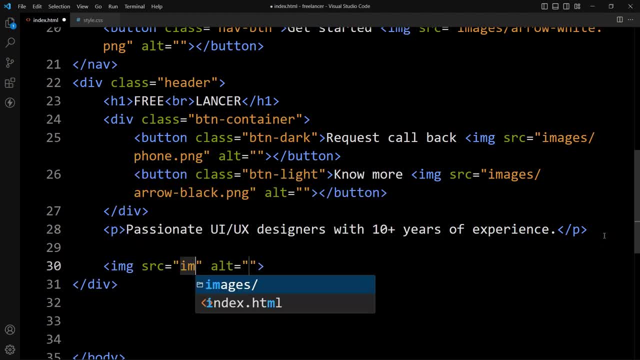 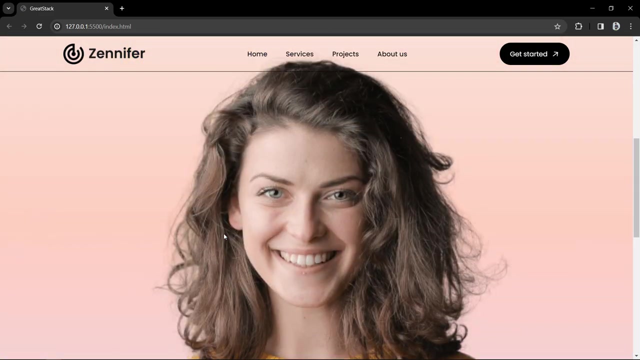 let's add header and p, add img tag, write the file path images, slash, user dot png. and in this one we will add the class name, user img. so we have this user img class name. after adding this, you can see we have this image here at the bottom. 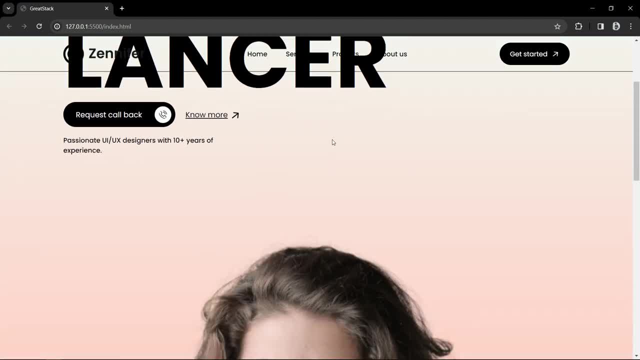 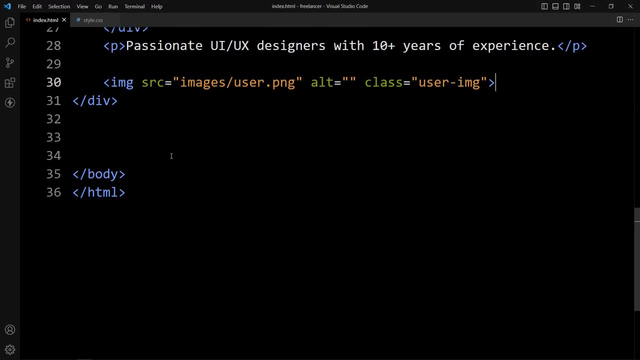 now, when i scroll the web page right, this text goes behind the navigation bar and they- these logo and menu links- are not clearly visible. so we will change the color of the navigation bar when we will scroll the web page. so let's fix this one first. so in this html file just above, 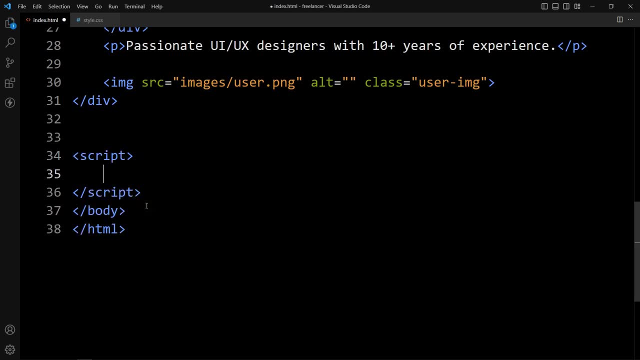 this body tag we will add a script and here we will add the javascript. so in this one let's add: window dot on a scroll is equal to one function, and here we have to change the color of the navbar. so first let's select the navbar. here we will add: let navbar is equal to document dot query selector. 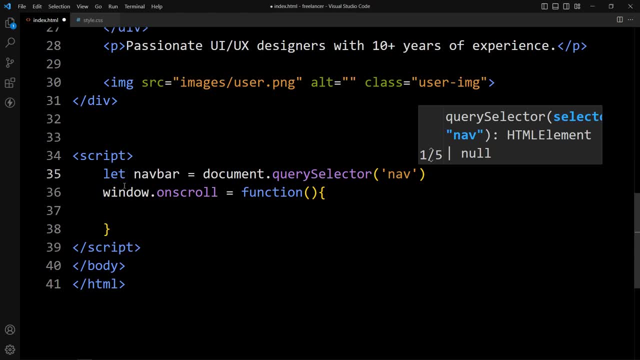 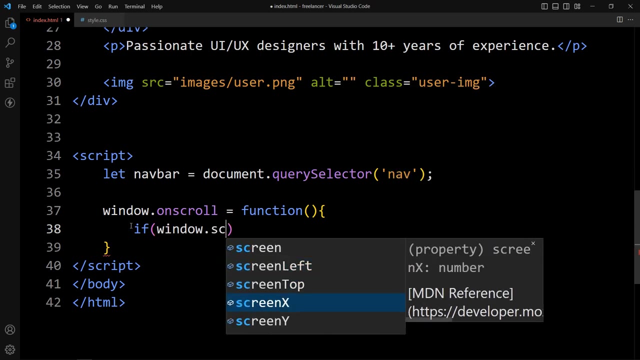 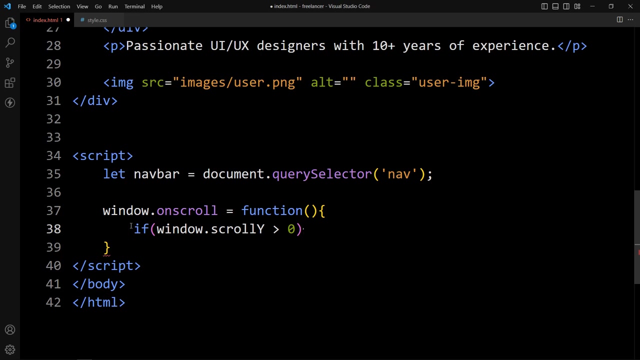 and in this one we will add nav tag. so it will select the navbar using the nav tag and here we will check the condition. we will add if, and we will add window dot scroll by if scroll y is greater than 0, it means we have a scrolled the web page. then what will happen from this navbar? 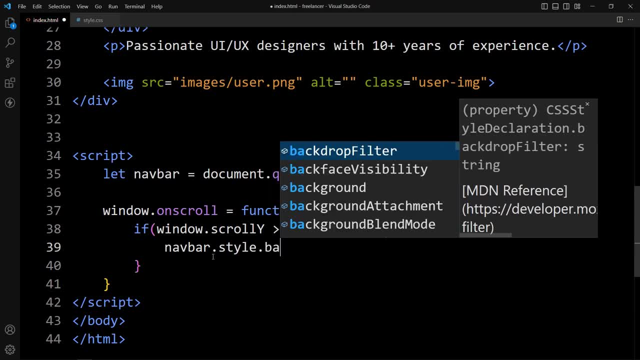 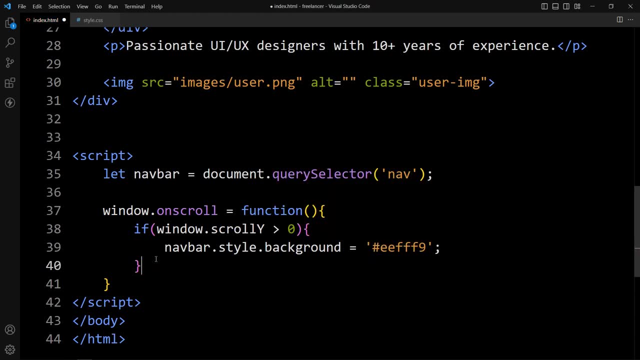 it will add style background and in this background let's add this color code and here we will add the else, if the window dot scroll by is not greater than zero, then what will happen? it will become transparent. so again, paste it and make it transparent. that's it. after adding this, you can see if i scroll the web page. 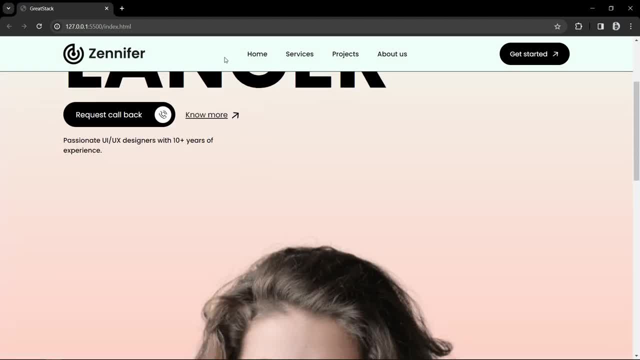 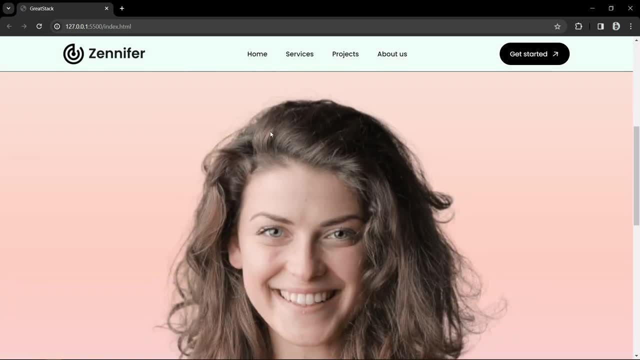 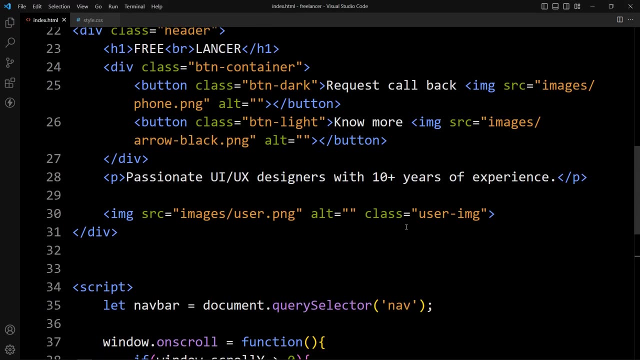 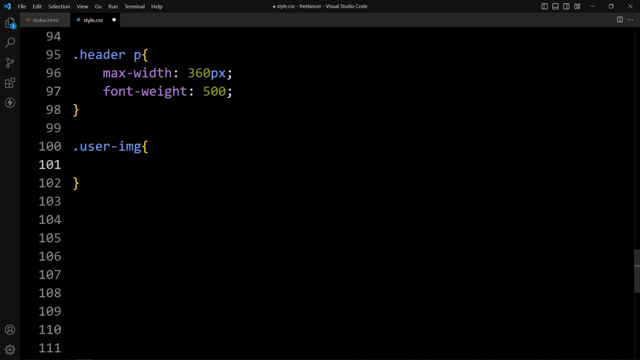 these links are clearly visible and this logo is also visible and this navigation bar is sticky at the top. now we will add the css properties for this image. so let's come back. and here we have added the user img class name. let's add this class name here in the css file. so for this user img we will add the width. that will be. 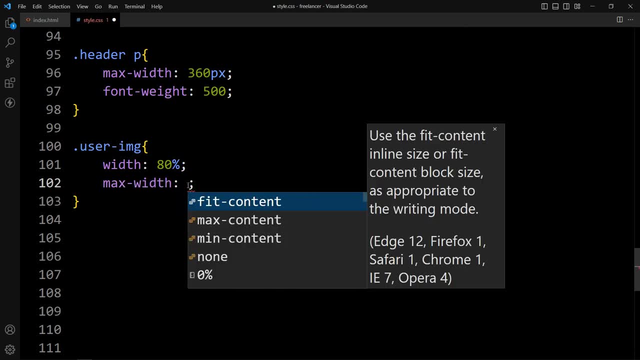 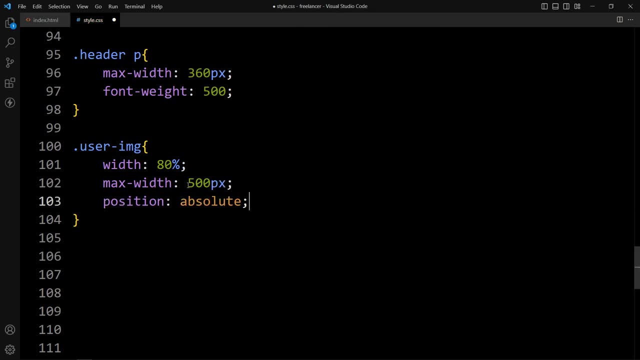 80 percent and we will add the map width. now the map within the isent门 crime area will be in maximum width, so the maximum width will be 500 pixel. then we will add the position absolute and right, so it will be in the right side. 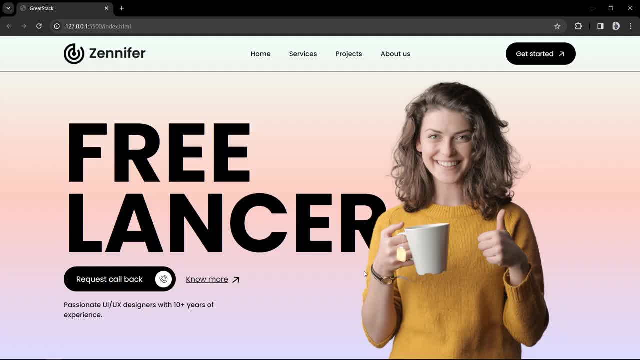 so it will be at 13, social space from the right side, and this image will be at the bottom. so we will add the bottom zero. that's it. after adding this, you can see the perfect position for this website header section. we will add the animation on this text. so we will add the animation in two. 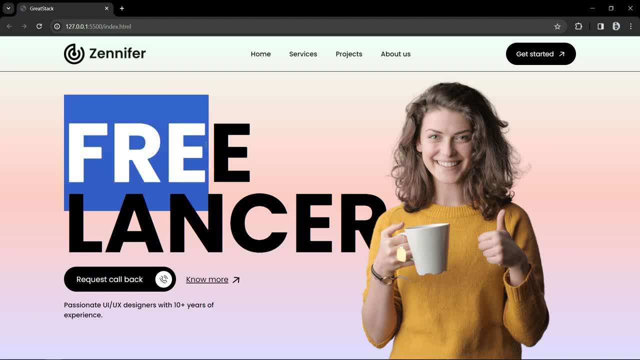 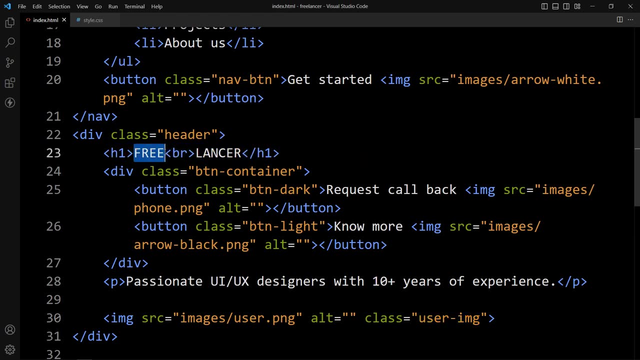 part. first it will animate the first line, then it will animate the second line. so let's come back to the html file. here we have this text in h1, which is freelancer. so here let's add one span tag, a span open and closing tag, and place this free inside this span, like this: now, after this break: 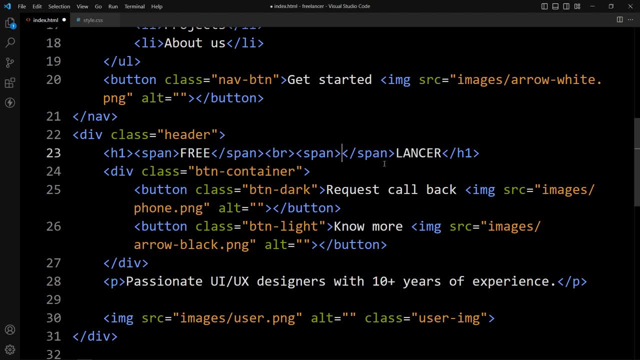 we will add again one span tag and in this span open and closing tag- we'll add the second line of text, lancer. so we have this first span tag, this second span tag. now we will add the css tag and we will add the css tag and we will add the css tag and we will add the css tag. 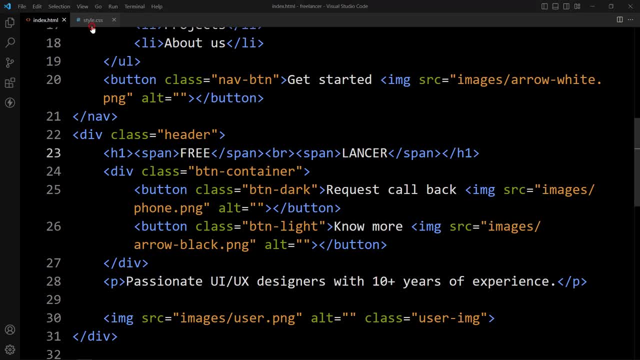 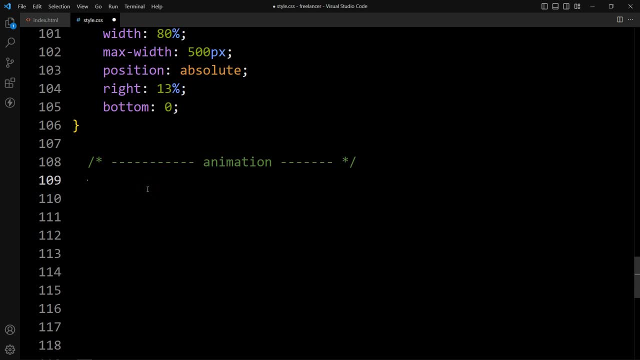 properties. so let's come back to the css file. here let's add one comment so you can understand from here i am writing the css for the animation. here we will add dot header h1 and span tag. let's add the background and in the background we will add linear gradient. 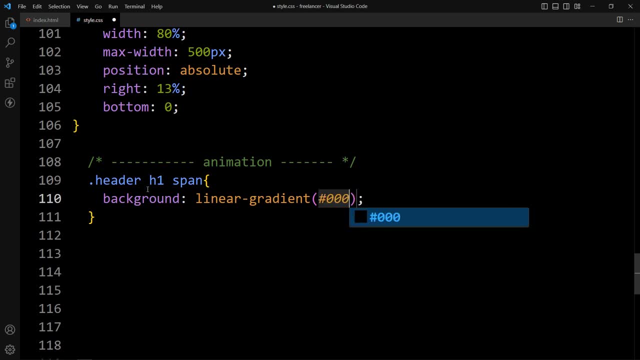 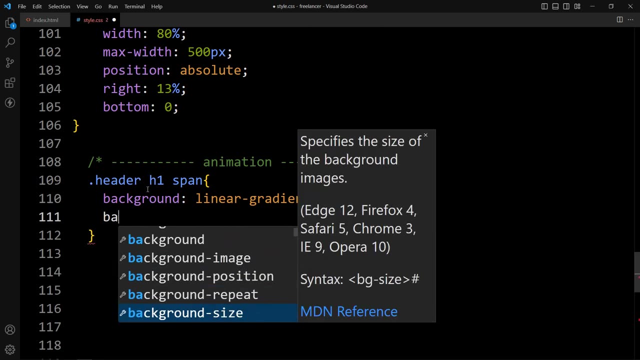 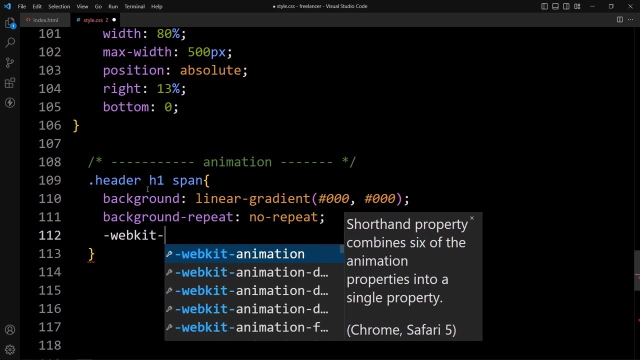 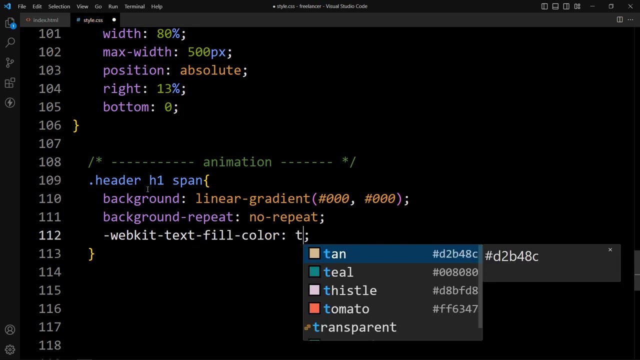 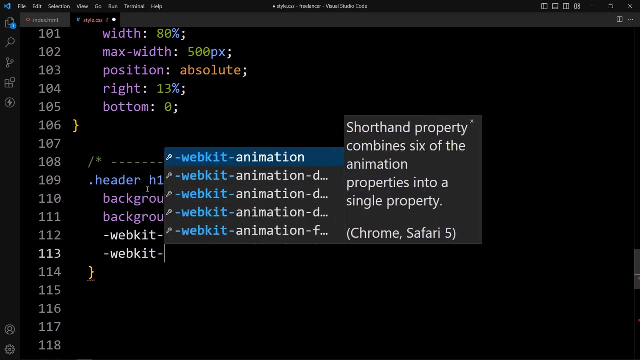 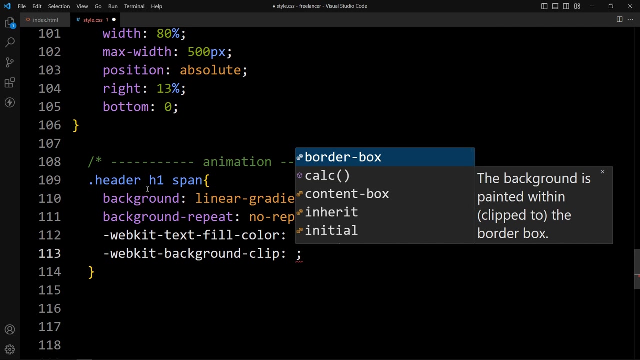 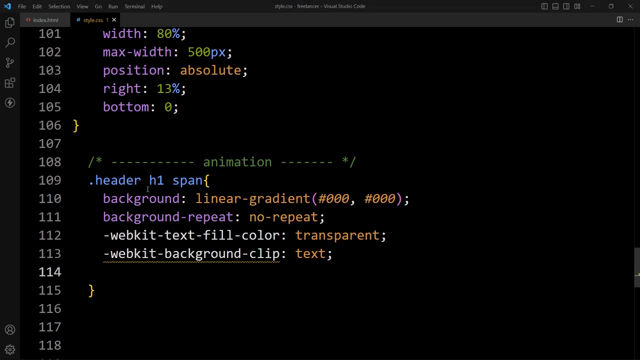 and the same color code, that is black. after that we will add the background- repeat, no repeat. then we will add webkit text fill color, so it will be transparent. after that we will add the webkit background clip. it will be text and after applying this you can see there is no change here. but if i apply background size, 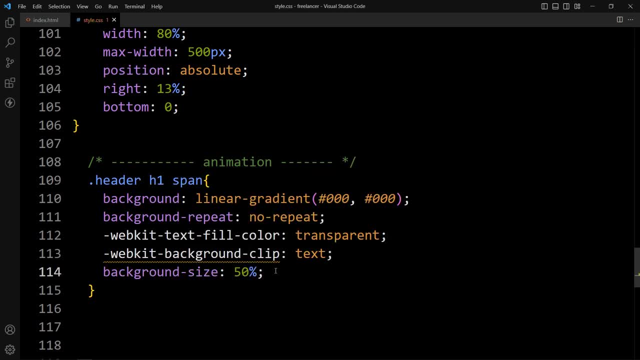 50 percent like this, so you can see only half text is visual from first line and second line. if i reduce- let's say 25 percent- from first line and second line: if i reduce- let's say 25 percent, you can see only 25% text are visible. if i make it 0: 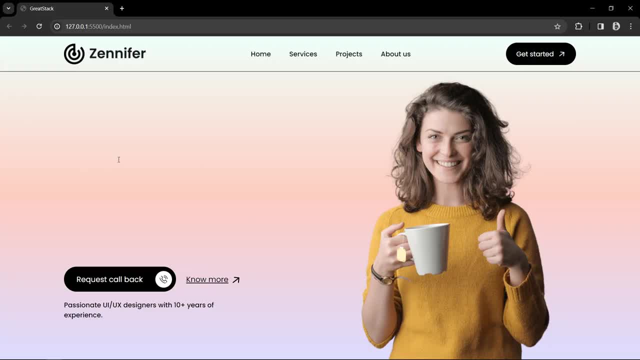 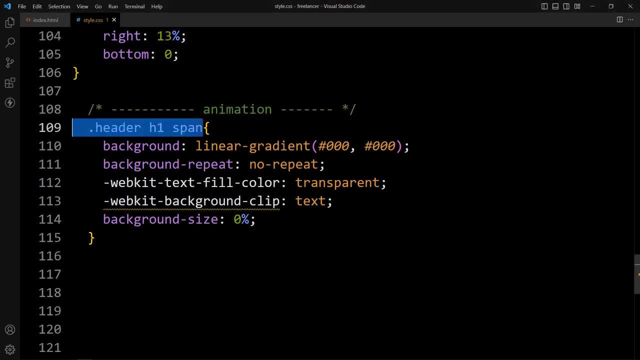 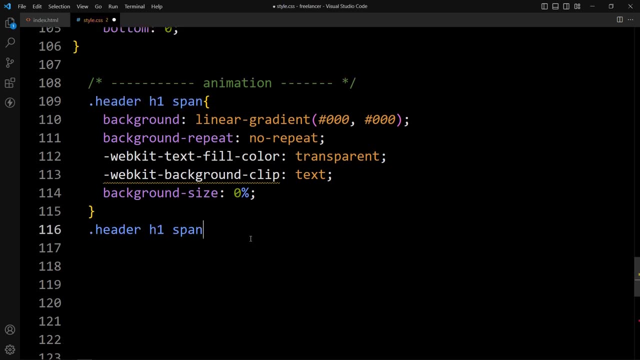 so the text is hidden. so we will use this to animate this text. so let's come back and here again copy this one, paste it here, and here we will add the css for the first span. so we will add first child that will select the first span only. so in this one we will add the animation. let's add the name of the animation. 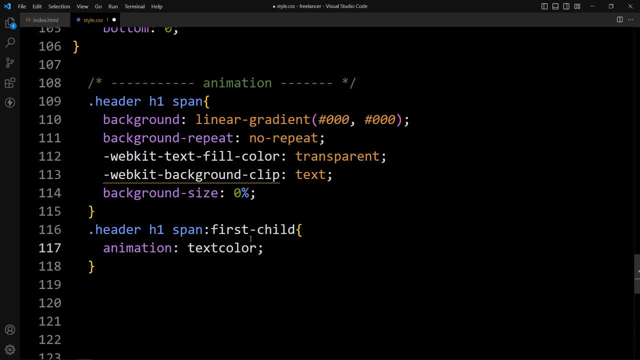 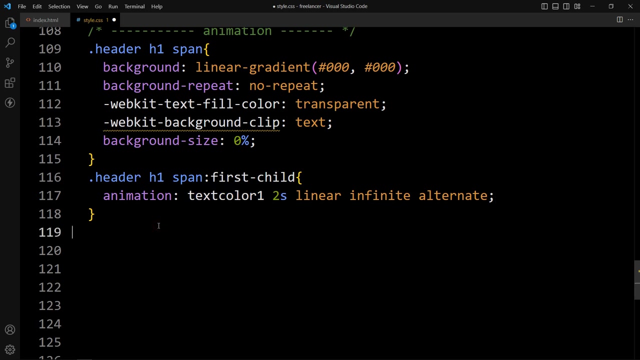 it will be text color one. this will be for two seconds, linear, infinite and alternate. it means first it will display the text, then it will hide the text using this alternate. now, after adding this, we will add the keyframes for this. so let's add the keyframes for this text color one here. 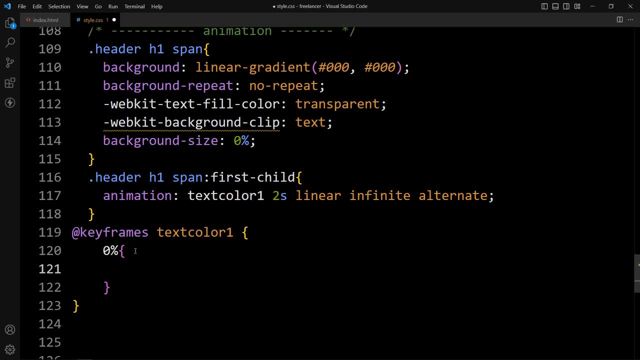 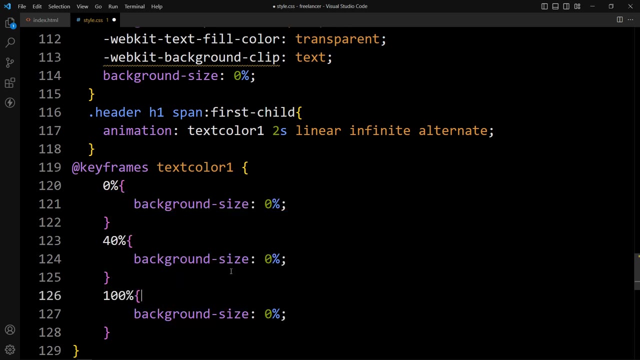 let's add zero percent, and at the zero percent this background size will be zero. now duplicate it, and here we will add 40 percent and 100 percent. so at 100 percent it will become 100 and at 40 100. so what will happen? initially, the background size will be zero. 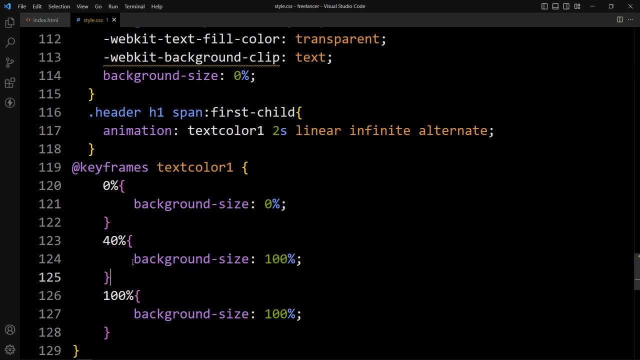 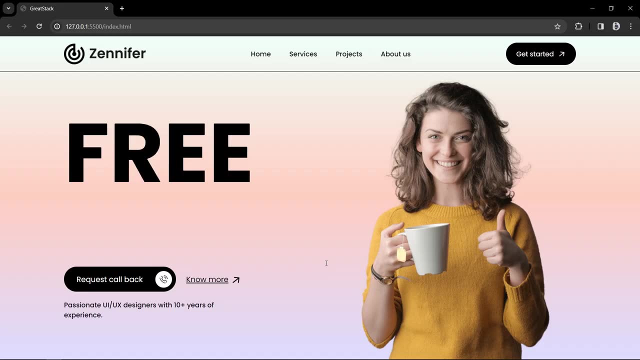 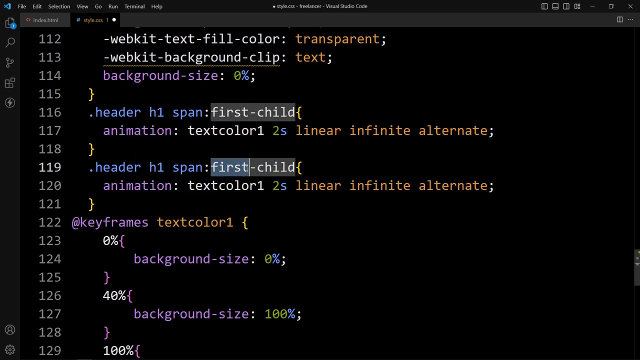 and after 40 percent time of this two. second, the background size will be 100, so you can see the animation in the first line. right now we will animate the second line, so here let's duplicate it, and it will be last child. here we have added first child. this is last child and here we will. 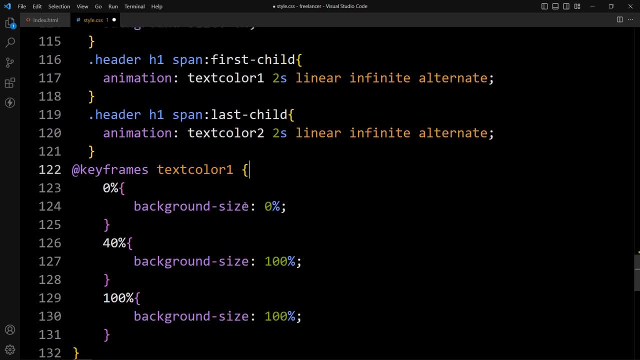 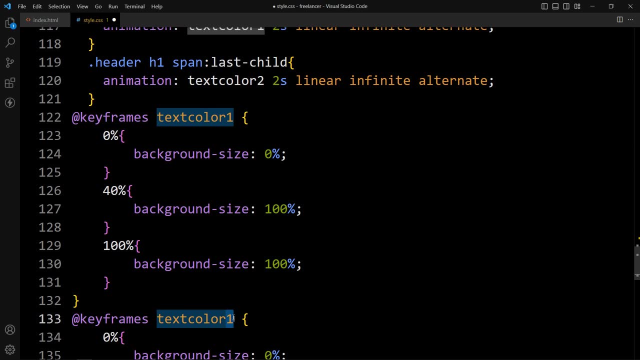 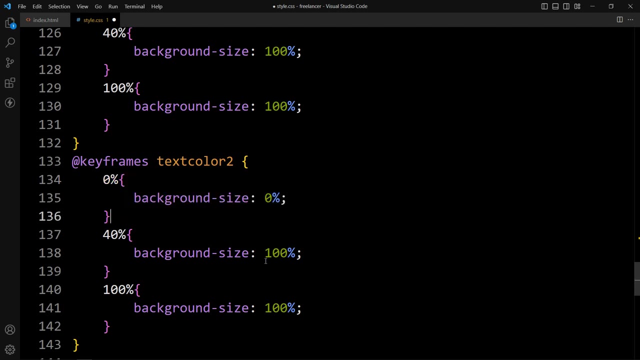 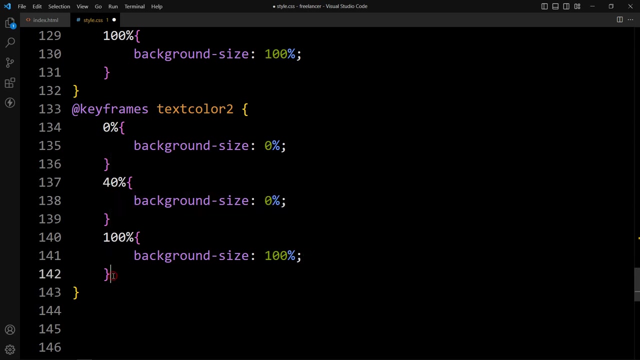 add text color two and we will add the keyframe for second one. so let me duplicate it. and here we will add text color two. in this one the size will be zero at zero percent, and here at the 40 percent it will be zero, and from 40 to 100 percent this size will increase, from 0 to 100. 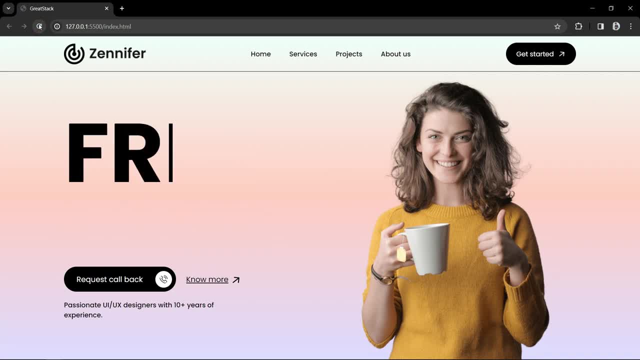 like this. so after adding this, let's refresh the web page. and now you can see both lines are animated. first it will complete the first line, then it has start animation in the second line. now we have created the animation also. next we have to make this web page. 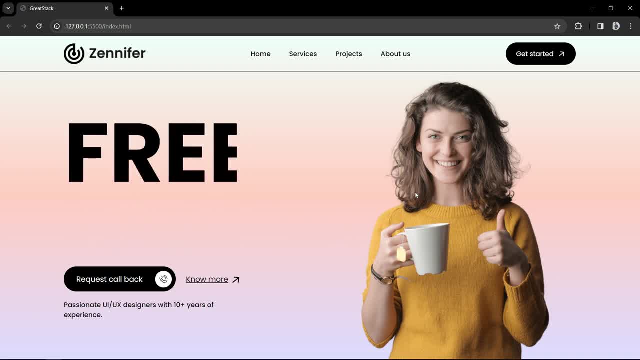 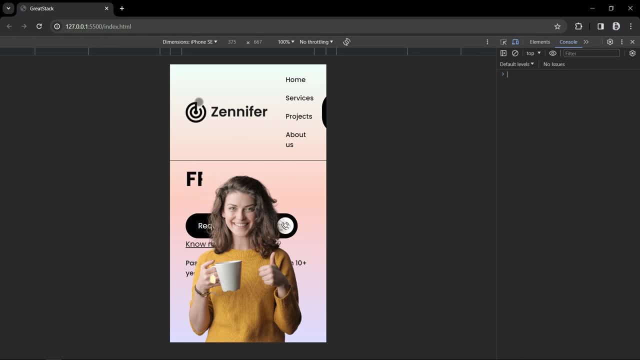 responsive for smaller screen. so let me change the screen size so you can see how it looks in the smaller screen. right now this logo is too big and here we have these links and button is not visible. so we have to remove this button and instead of that we will add one menu icon. 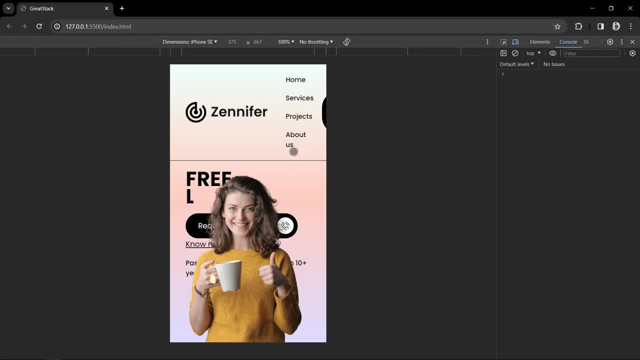 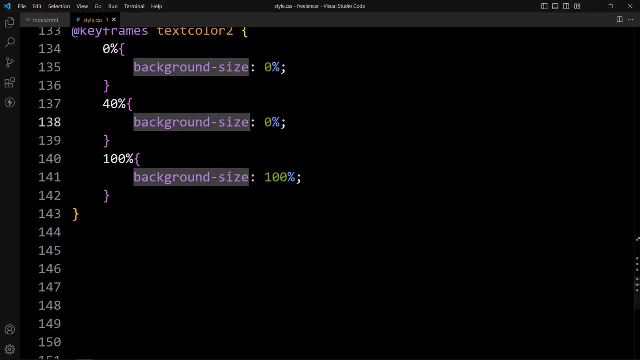 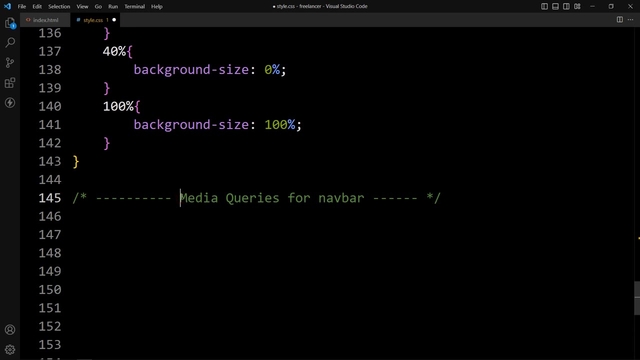 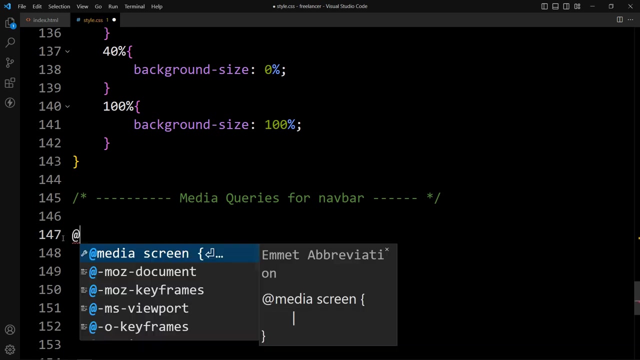 and these menu list will be hidden. it will be displayed when we will click on the menu icon. so let's come back here. in this CSS file, here let's add the comment. so here you will understand. I am adding the media queries for navigation bar or navbar. so in this one let's add, at the rate, media only, screen and max width. 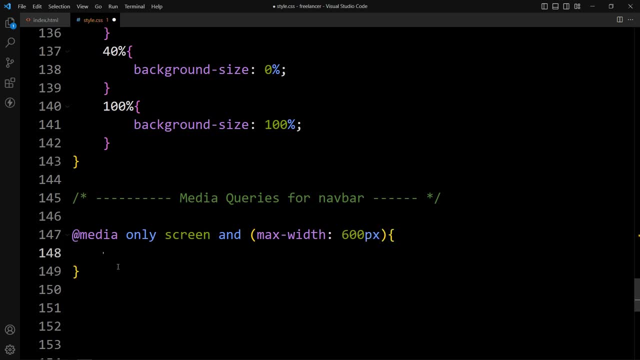 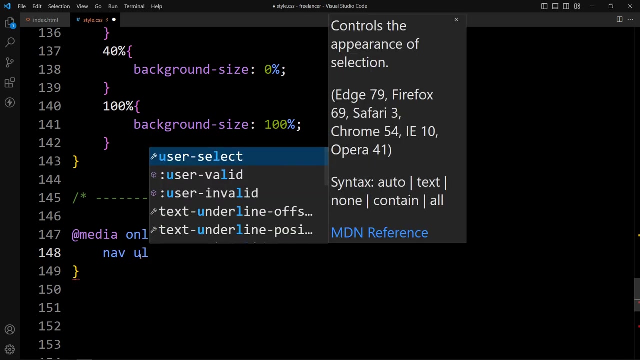 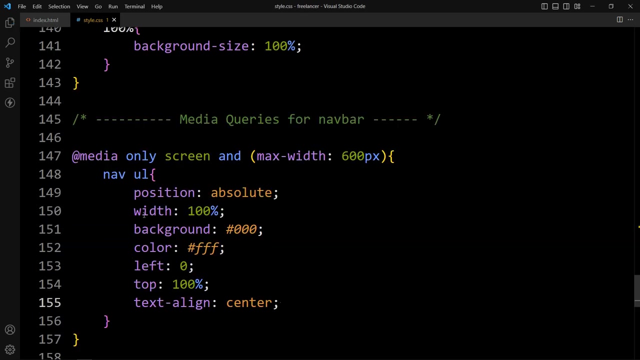 600.. so within this media query we will add the CSS properties that will be applicable for the smaller screen whose width is less than 600 pixel. so here we'll add the nav ul like this and we will change the CSS properties. so in this ul we have added the position absolute. 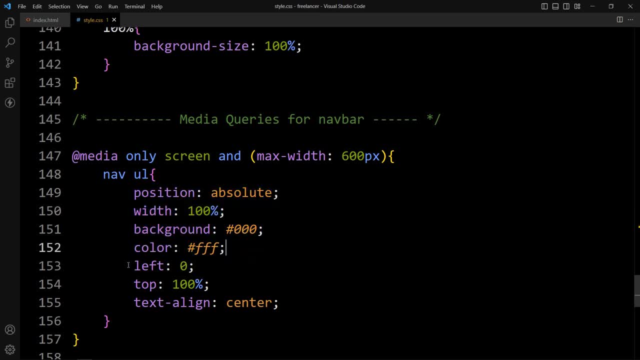 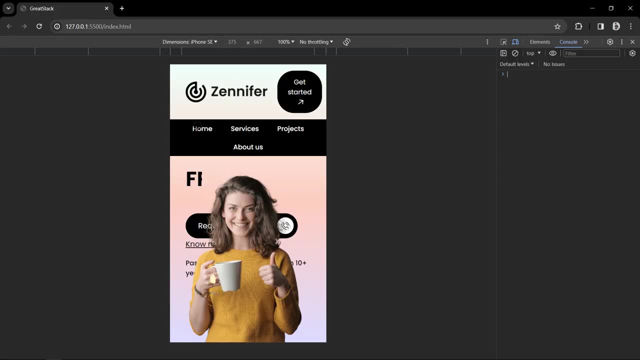 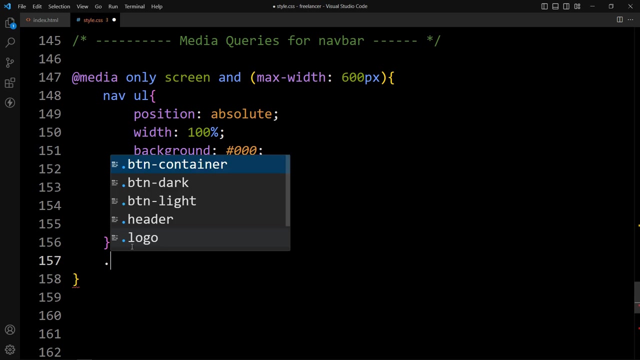 width hundred percent. added the background and color left zero top hundred percent. text align center. so you can see this menu links are displaying just below this white navigation bar. after that we have to hide this button. so let's come back and here we will add dot nav btn display none. then we have to change the size of the logo, so we will add nav dot logo. 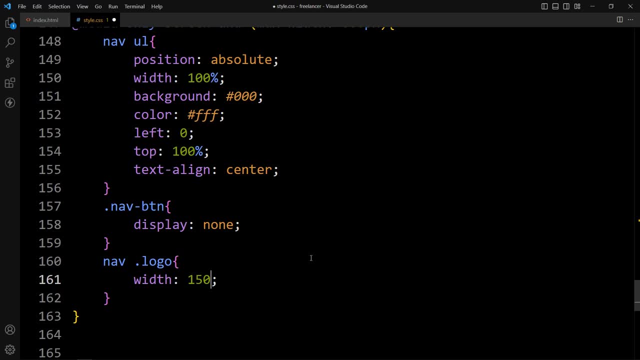 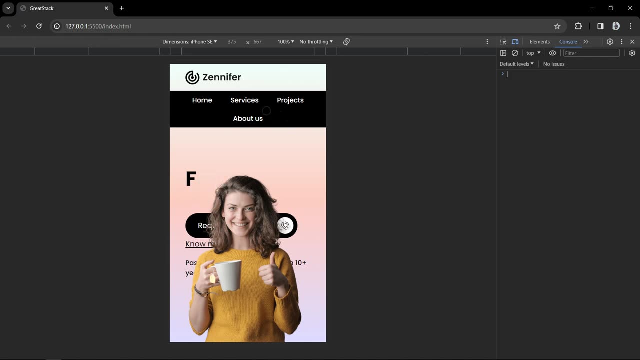 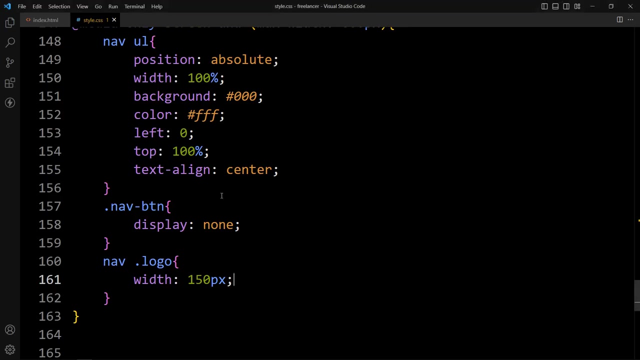 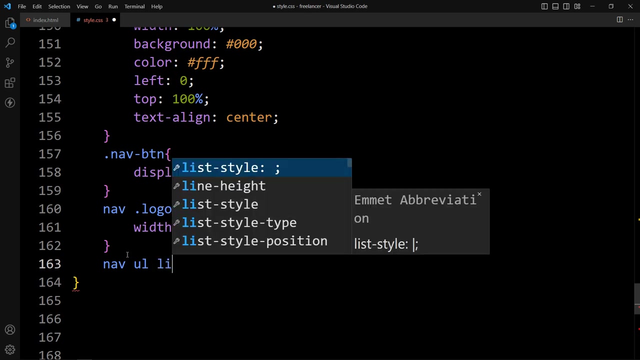 so let's decrease the size. width will be 150 pixel. so here we have the logo only and these links. now we have to decrease the space between these links so it will come in the single line. so let's come back. and here we have the CSS for nav ul. so let's add the list also. so nav ul li. so for these list we will add the margin. 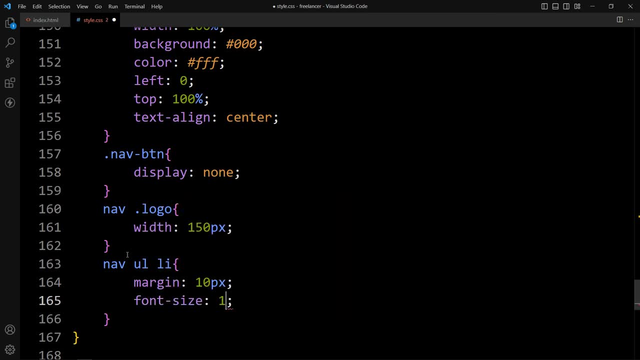 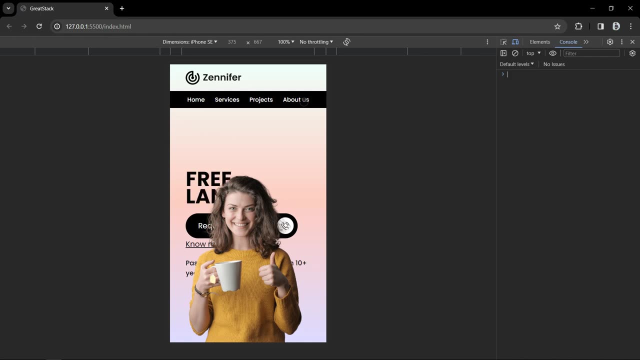 10 pixel and we will decrease the font size 14 pixel. now it is coming in single line. after that we have to add one menu icon. using that icon, we can display or hide the menu links. so let's come back to the HTML file, and here we have this button. so after this button, we will add: 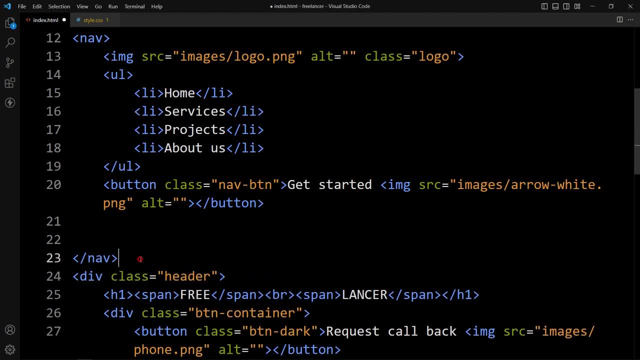 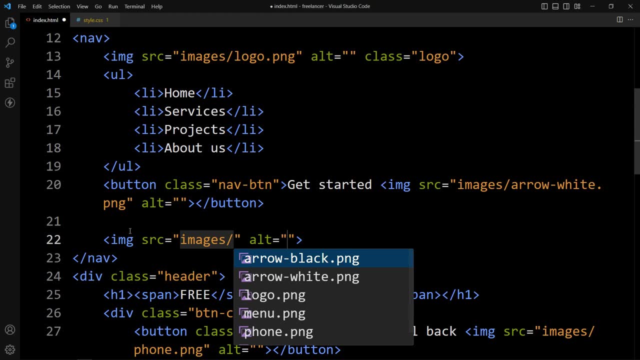 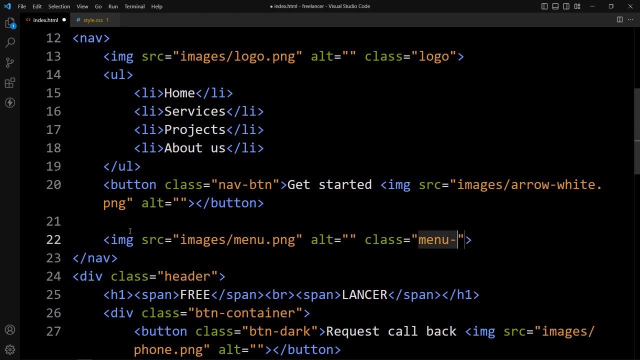 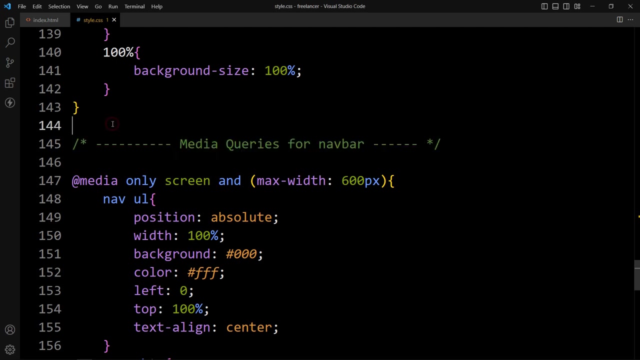 one icon. so here, above this closing nav tag, we will add img tag. write the file path images, slash menu dot png and we will add the class name menu icon like this: save this and come back to the CSS file above this media query. media query is starting from here, so here let's add. 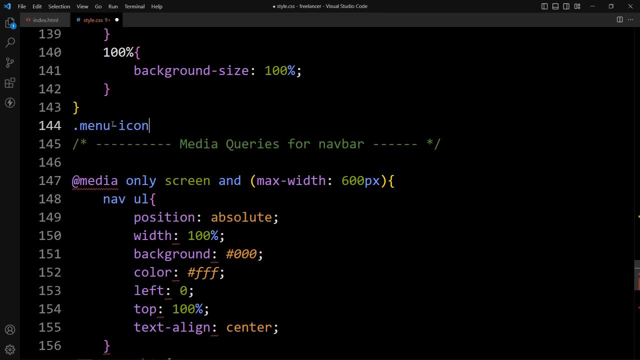 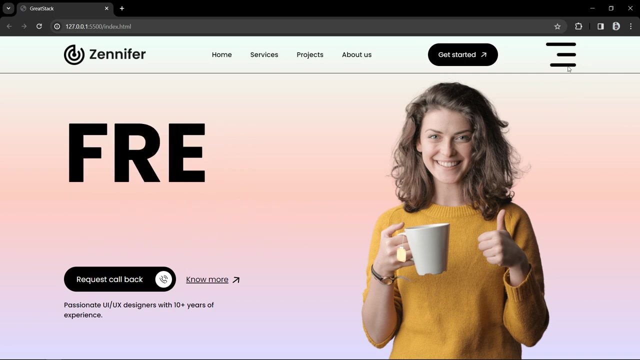 that menu icon dot. menu icon display none, so this menu icon will be Hidden. if I come back to the webpage and open this in full screen, you can see there is no menu icon. if I remove it, you can see this menu icon is visible on the desktop screen also. that's why here I'm adding 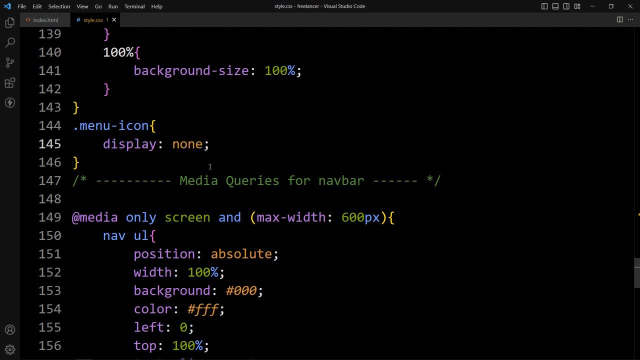 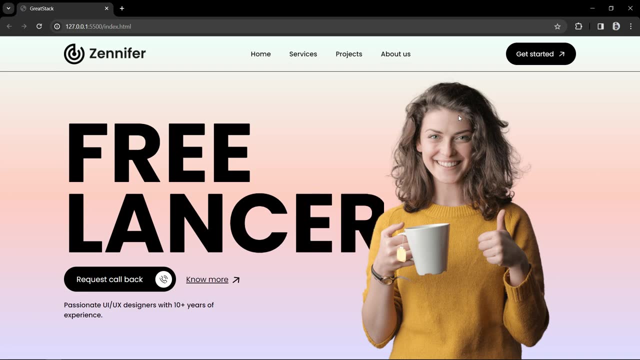 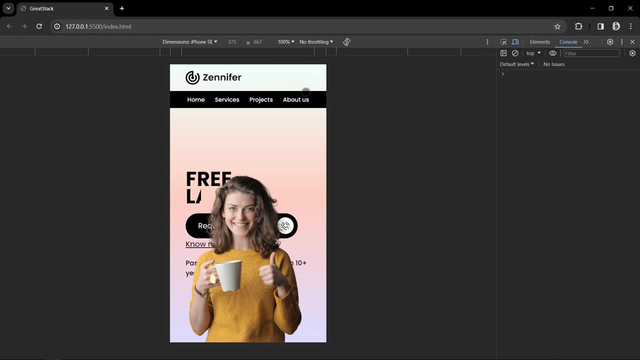 display none outside of the media query, so it will hide it from full screen. let's open it in the smaller screen. so in this, a smaller screen, you can see still, menu icon is hidden, so we have to display it in the smaller screen. so let me come back and here we'll add this menu icon. 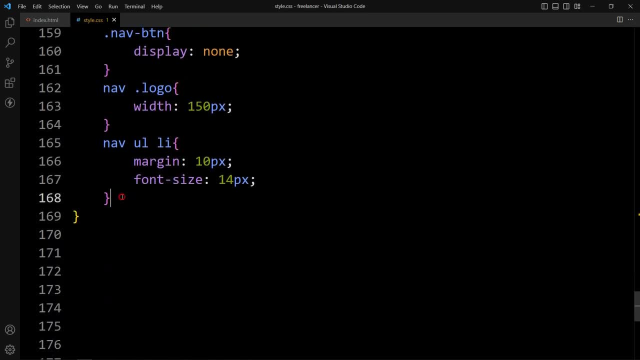 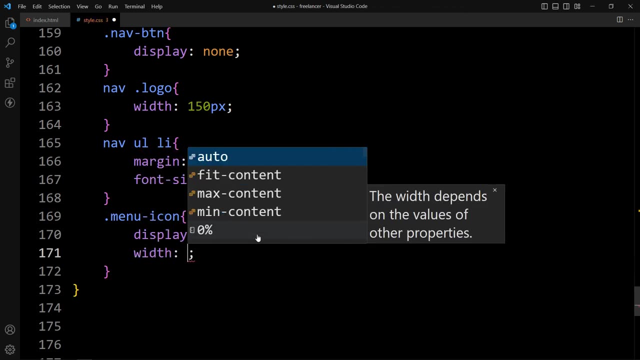 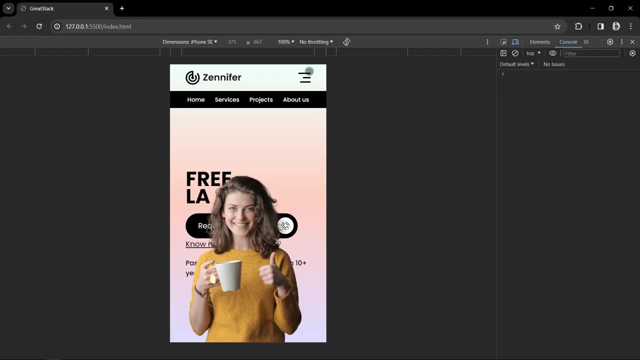 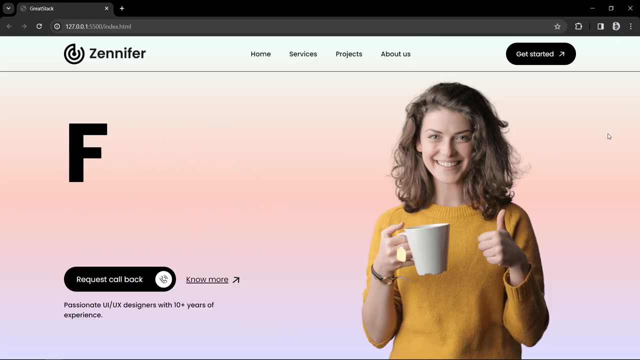 in this media query, menu icon display will be block and width will be 30 pixel, so you can see the size for this menu icon is perfect and it is visible on a smaller screen, and when we open it in full screen, the icon is hidden and it is visible in smaller screen. next, 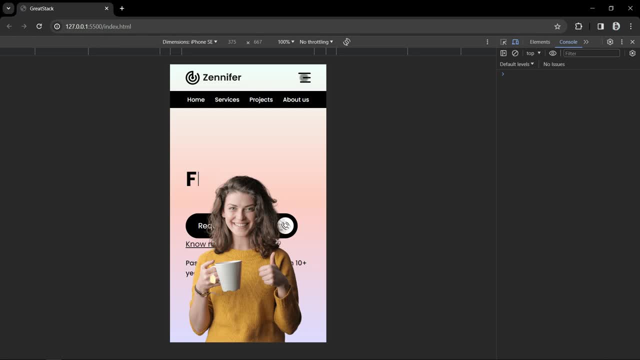 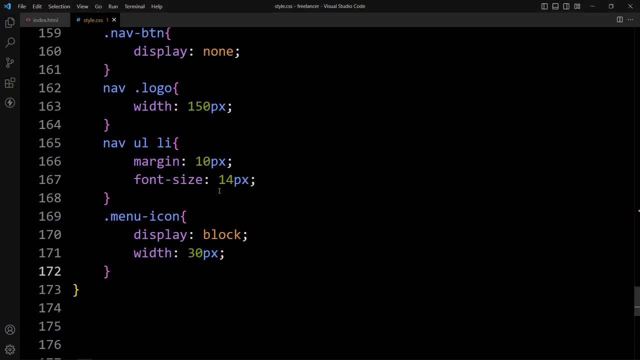 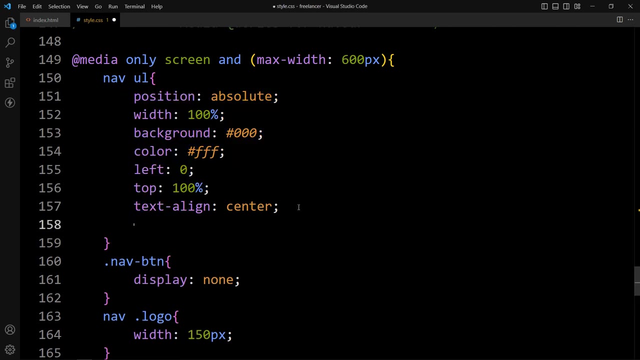 we have to add the click feature on this menu icon so that it will hide or display this menu links. for that let's come back, and here you can see we have ul. so in this one we will add the max height- max height: 0 and we'll add the overflow hidden, so the links will be hidden. 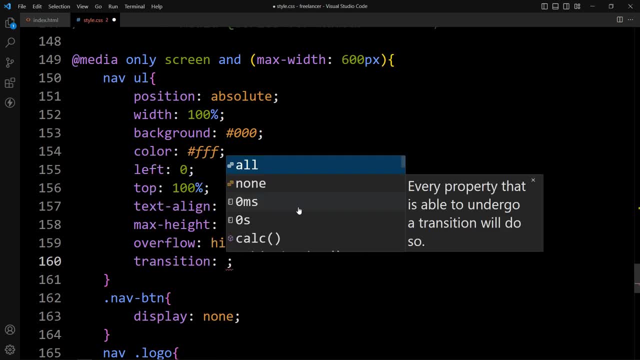 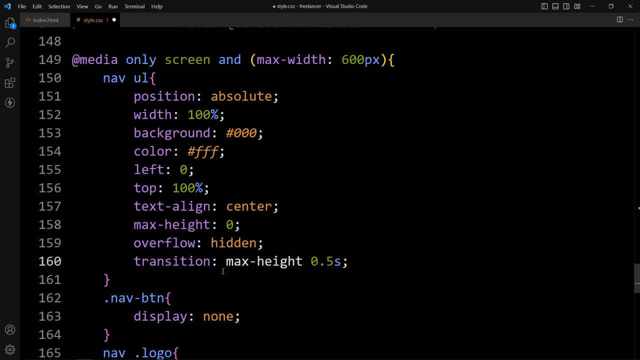 and here we'll add the transition also. transition of max height: 0.5 seconds. so when we will increase the max height, the links will be visible again. so after adding the links, adding the max height 0, you can see these links are hidden. next we have to. 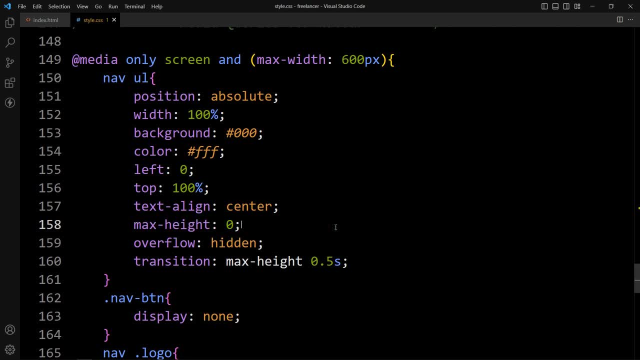 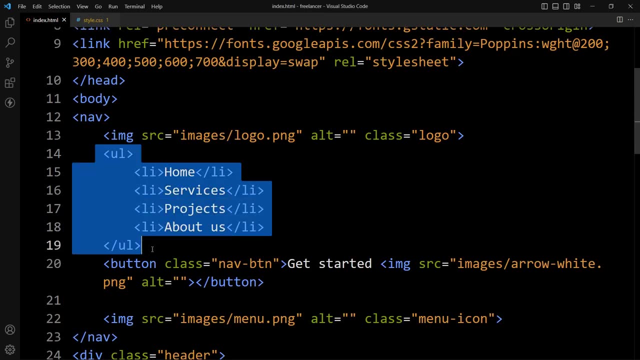 increase this max height using JavaScript whenever we will click on the icon. so let me come back to the HTML file. so we have to increase this height of this ul. so in this one let's add one ID. we will add the ID menu links like this, and we have to add the click feature on this menu icon. so on this, 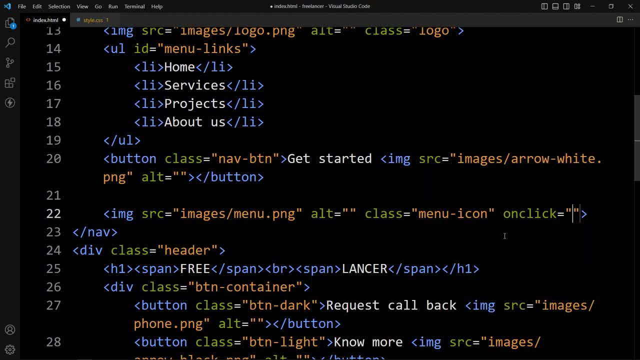 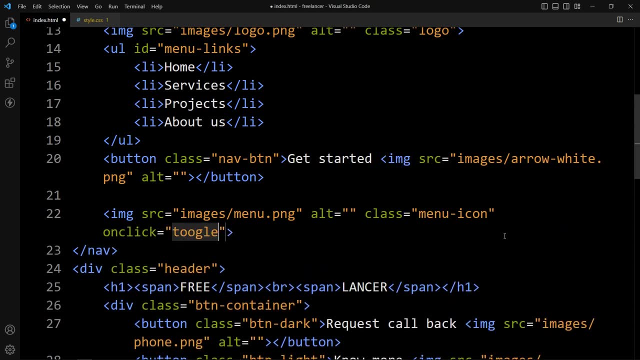 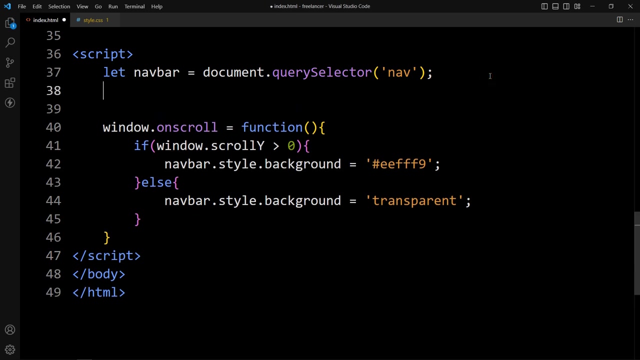 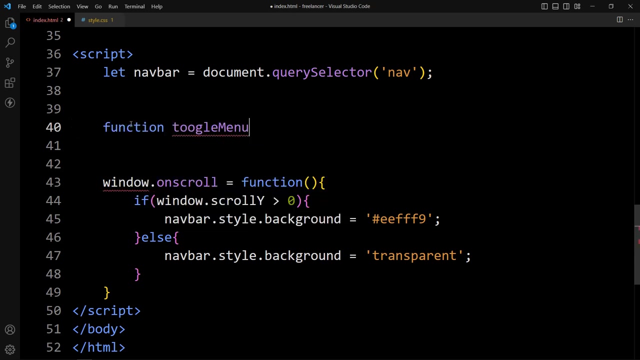 menu icon will add on click and call one function. let's say toggle menu. here we are calling toggle menu function, so let's define this toggle menu function. so in this JavaScript here only we will add space and let's add function toggle menu like this: and we have to select that ul. so let's add let menu links is equal to document dot. 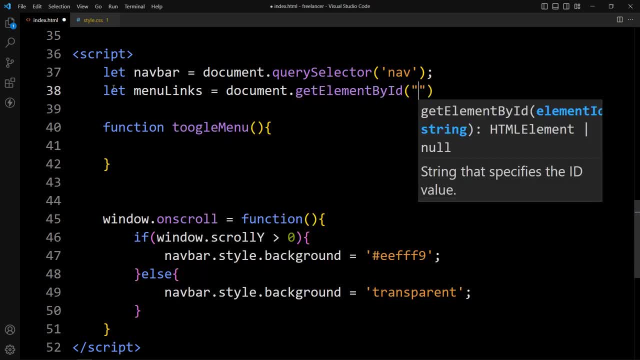 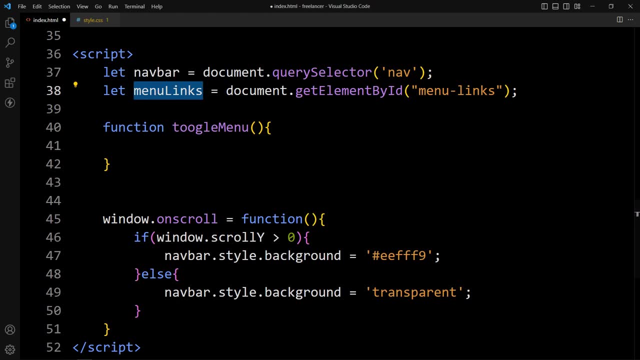 get element by ID and place the ID that we have just inserted in the ul tag. so we have selected the menu links. now for this menu links we have to add a new class name or remove the class name. so we will add menu links, dot, class list, dot toggle, and here let's add a new class name. that 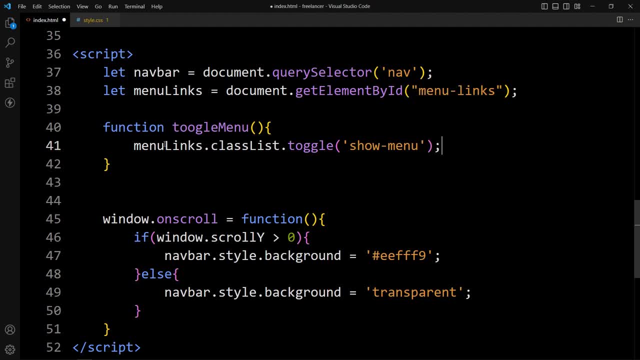 is so menu. so what will happen? whenever we will click on the menu menu icon, it will execute this toggle menu function and this toggle menu function will select this menu links. that is a ul tag, and in that one it will add this recycling class name and if it is already there, it will remove. 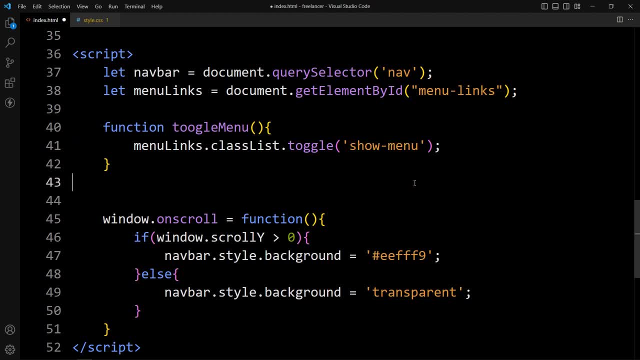 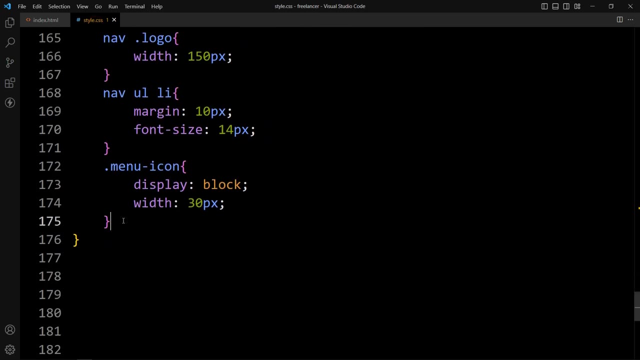 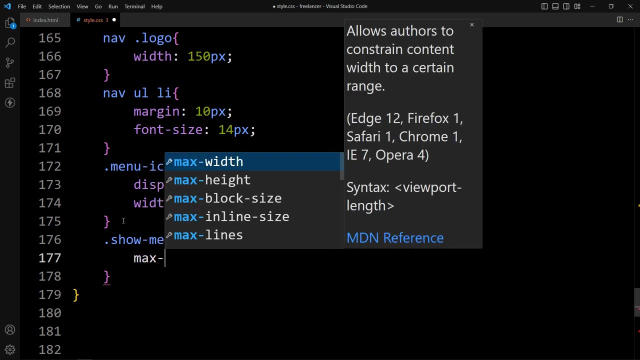 that class name. that means when you will click the first time, it will add the class name. when you will click again, it will remove the class name. so let's add the CSS properties for this new class name. that is so menu. so what will happen? we have to increase the max height. so just add so menu. and here let's add max. 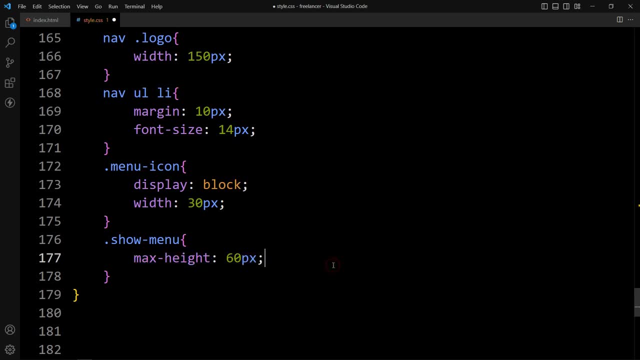 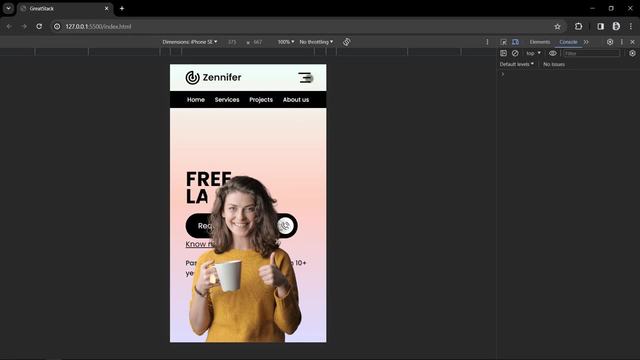 height of 60 pixel. that's it. after adding this again, come back to the web page and let's click on this menu icon so you can see it display the menu links with smooth animation. let's click again. it will hide the menu links so you can. 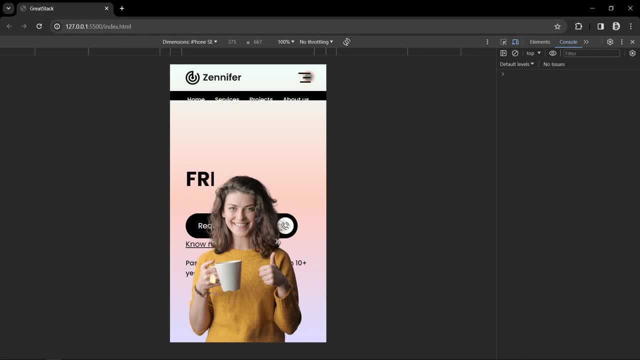 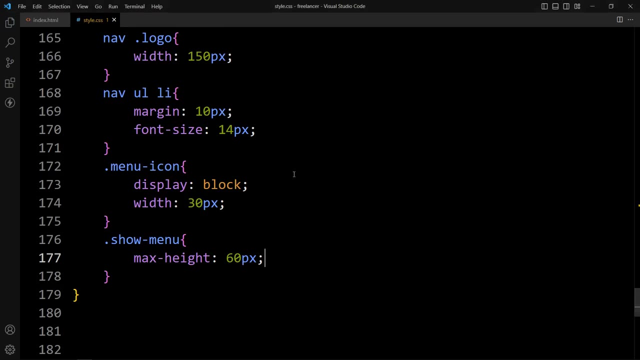 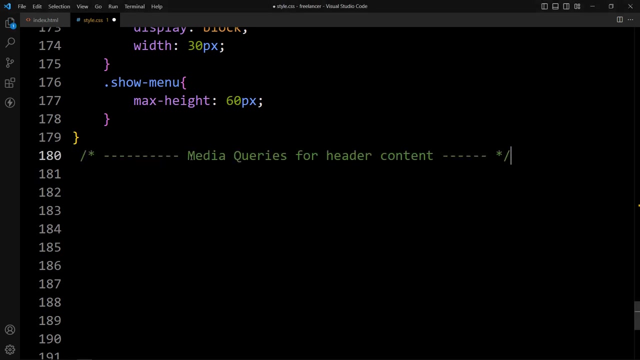 see this toggle menu is working fine for this: a smaller screen. next we have to add the CSS properties for the header content, which is the text and this image. so let's come back to the CSS file and here let's add the comment again, and here I'm adding media queries for header content. you can add the media queries. 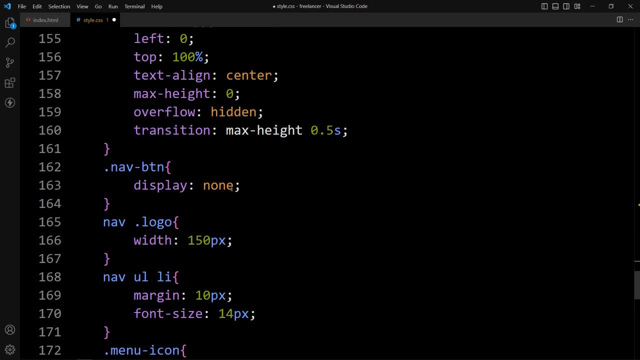 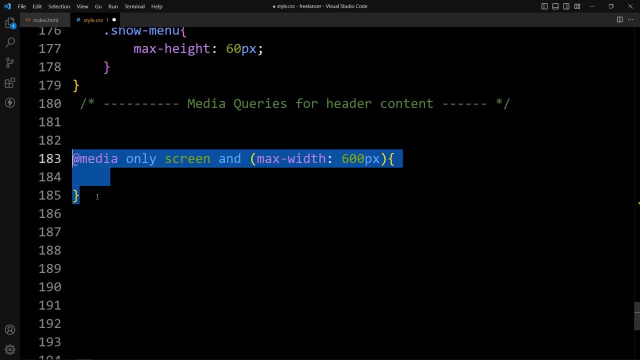 here only, but you can add the media queries here only. but I am writing it separately so you can understand it clearly whenever you will open the code file. so here again we'll add another media query and here let's add dot header, and in this one we will add min height auto. earlier we have 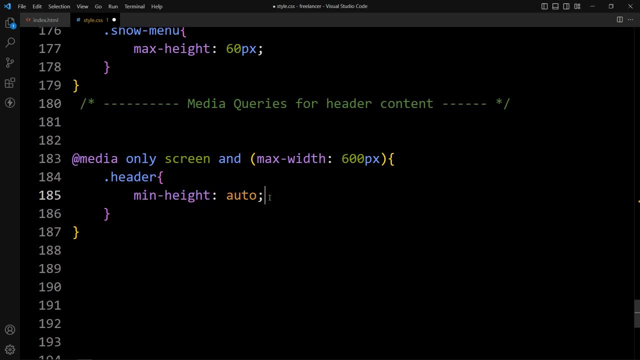 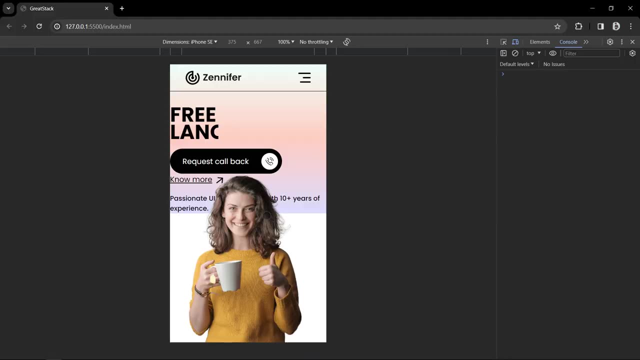 added min height: 100 VH. so we will set it auto for small screen and we will remove the padding. also, the padding will be 0. after removing the padding, you can see these text are coming from the left side. right now we will add the CSS properties for this user image, so 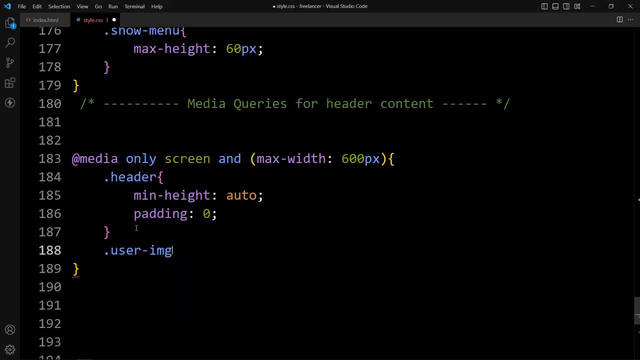 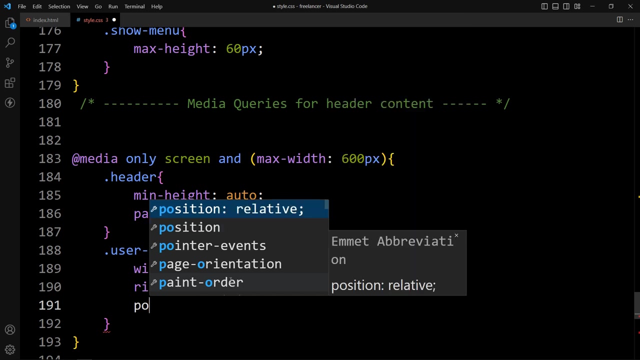 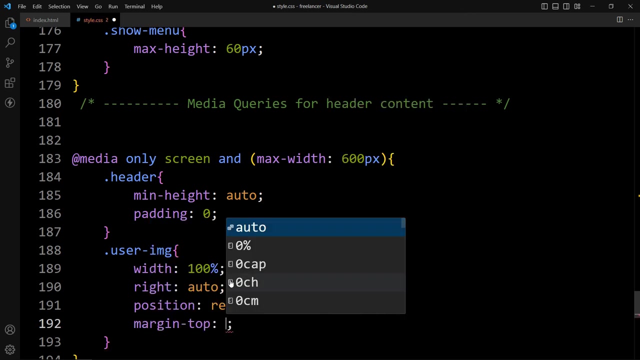 here. let's add dot: user image and width will become 100%. then right otto. earlier we have added the right like 13%, so we will set it or we can set auto and we will add position relative. after that we will add margin from top. that will be 100 pixel. so after adding this CSS for the user, 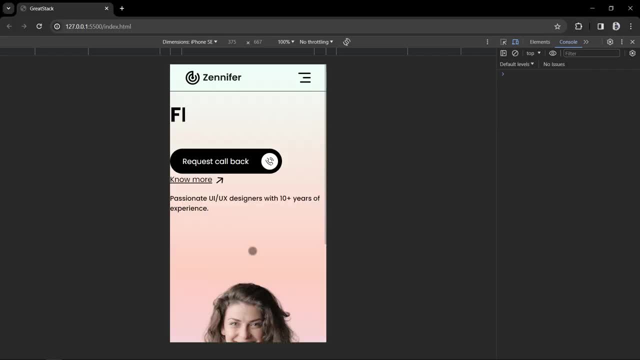 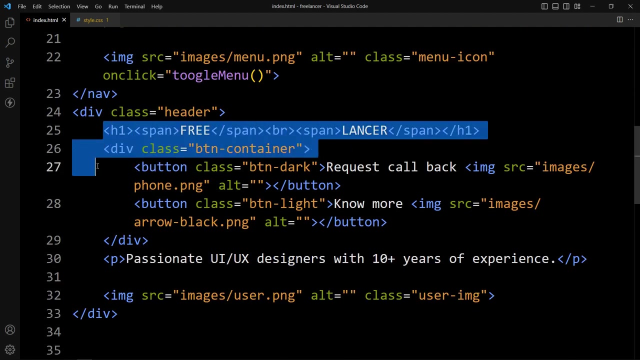 image you can see. it is coming here right next. we have these content here, so we will insert all these text buttons and this paragraph text in one div so that we can set the position at the bottom. so let's come back and here in this HTML file we have this h1 text, then these buttons and this paragraph, so we 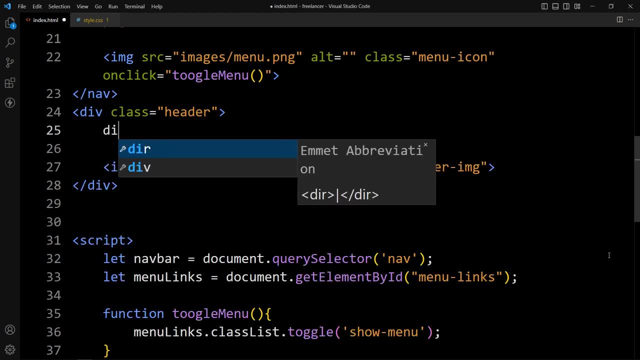 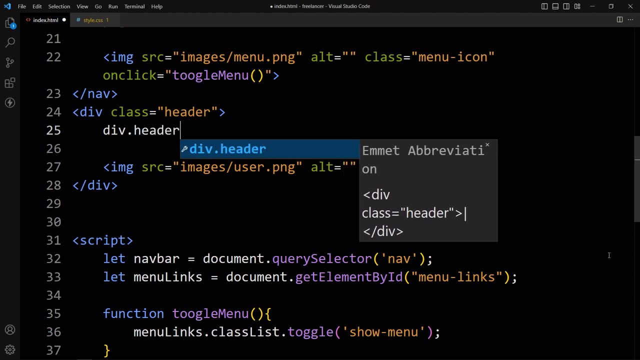 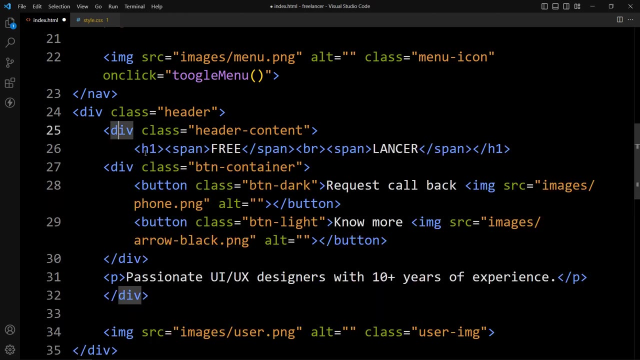 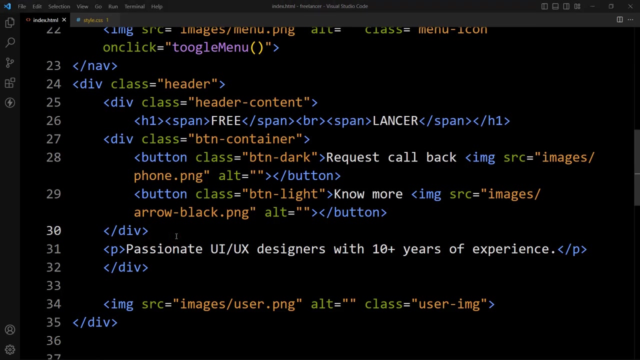 will insert all these things in a div. so here let's add one div and let's say: the class name is header content and here, in this header content, we have inserted this title, this button and this paragraph text. after adding this, you can see there will be no. 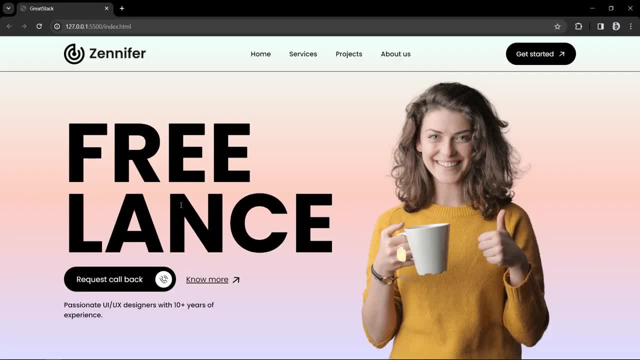 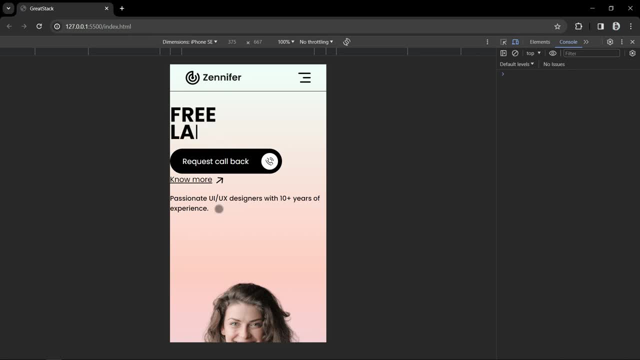 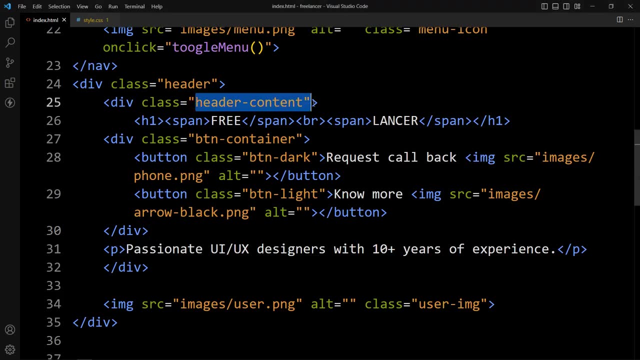 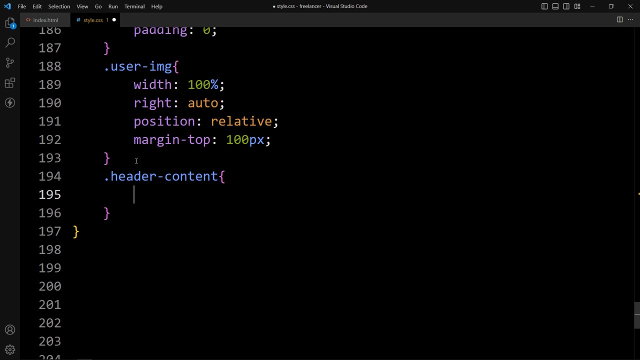 changes here and there is no changes on full screen also. but we can add the CSS using that new class name for all these text button and this paragraph. so let's go back and copy this class name, header content, place it here in this media query and for this one we will add the CSS properties. 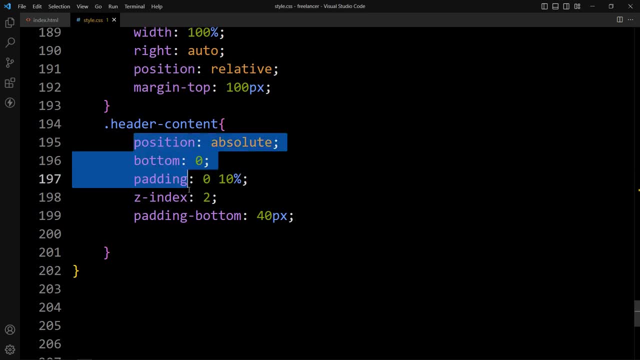 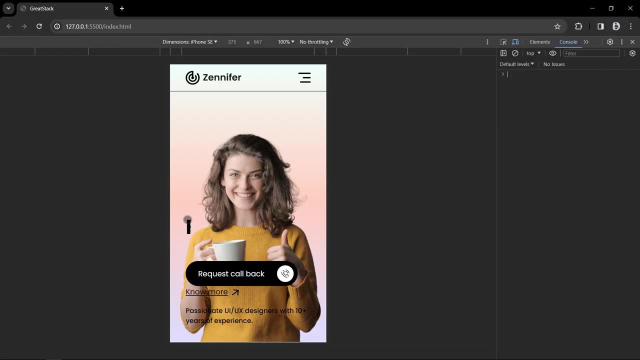 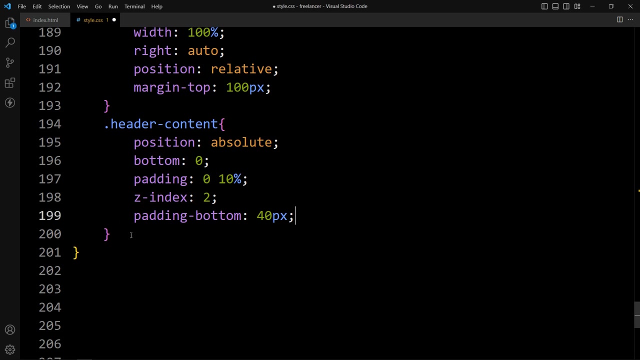 so after adding these CSS properties- position, absolute bottom, padding z index and padding bottom, so you can see the position for this text and button is perfect. next we have to add the CSS for this button. so let's come back and we will decrease the space. so here let's add that class name dot, btn container, and in this one we will add the 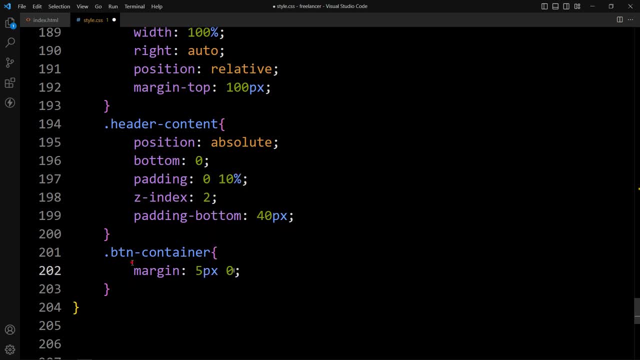 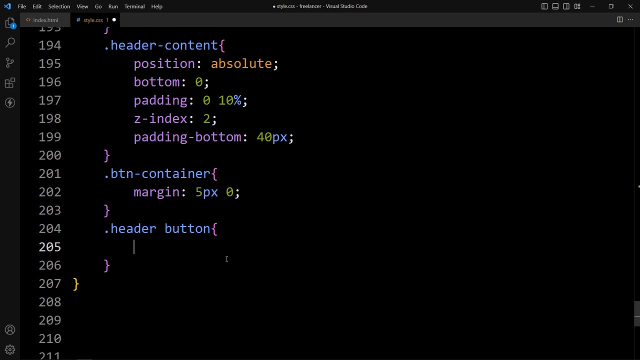 margin of 5 pixel 0. earlier it was 20 pixel and 0. after that. for the individual buttons we will add the CSS. so here we will add dot header and button. so for this button we will add the font size. that will be for both buttons and margin right. 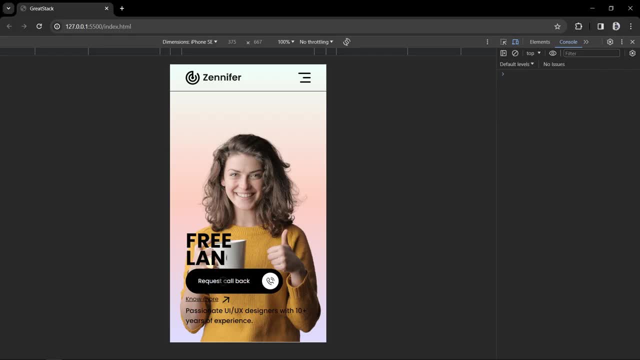 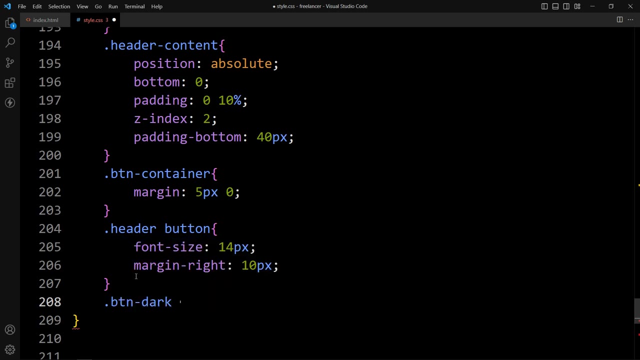 10 pixel so you can see the changes in the space and font size of the button. after that we will add the CSS for the dark button. so let's add dot dark and here we'll add the padding. we will decrease the padding and we'll add the margin bottom. 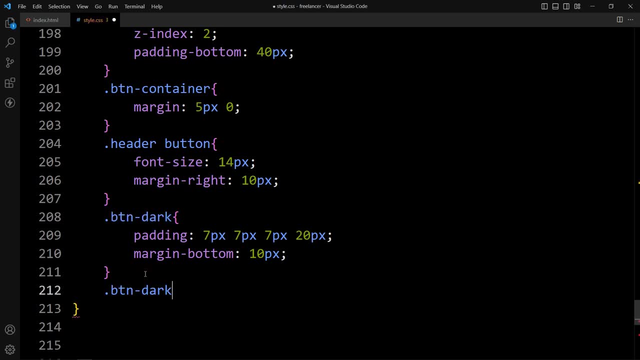 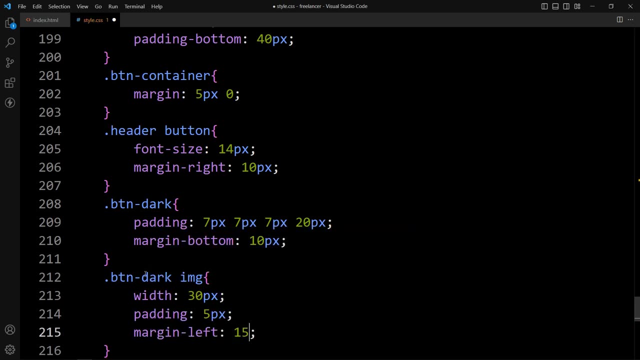 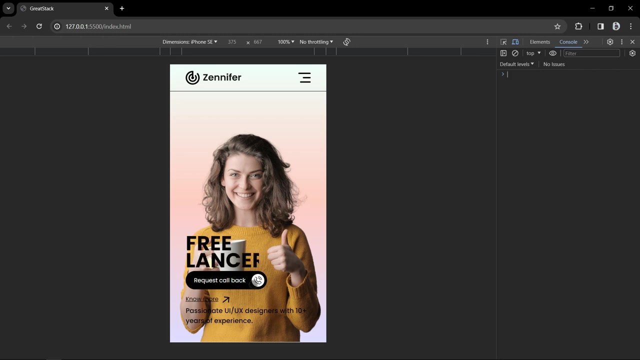 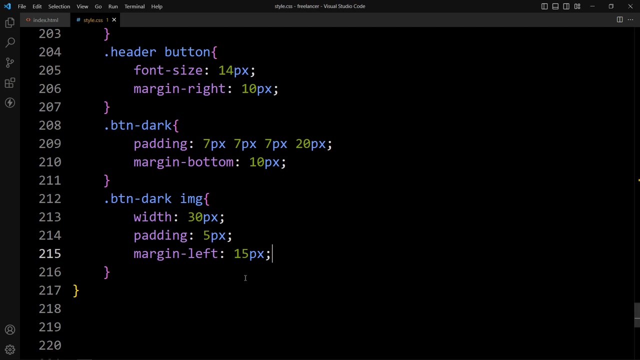 and in this dark button we have one icon also. so let's add the img tag and we will decrease the width. so after adding the CSS, you can see the size for this request. call back button is perfect. next we will add the CSS to decrease the size of this arrow icon for the second button. so for the second button, the class name is: 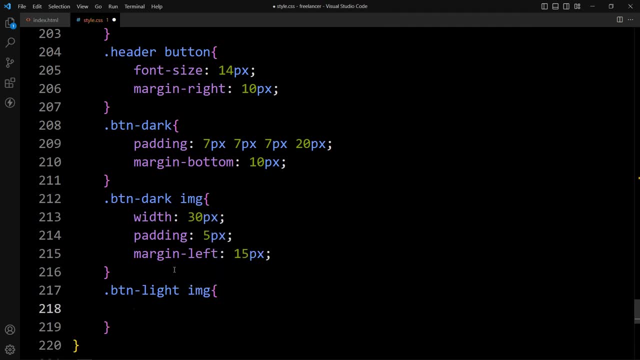 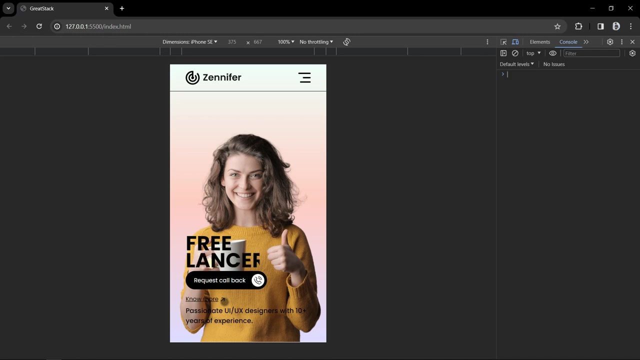 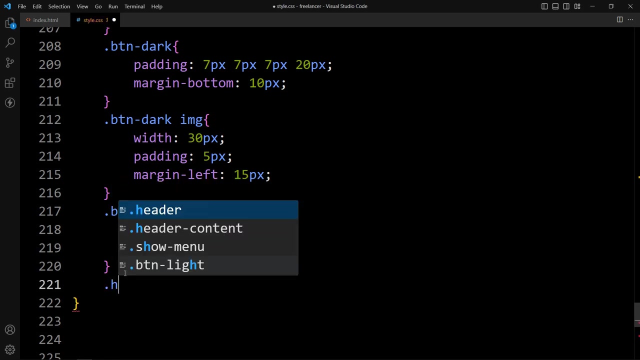 btn light and write the img. here we will decrease the width and margin left, so the size for this icon is also good. next we have to increase the size for this font. let's come back and here we'll add dot header h1. so for this h1 we will add the font size of 70 pixel and line height. 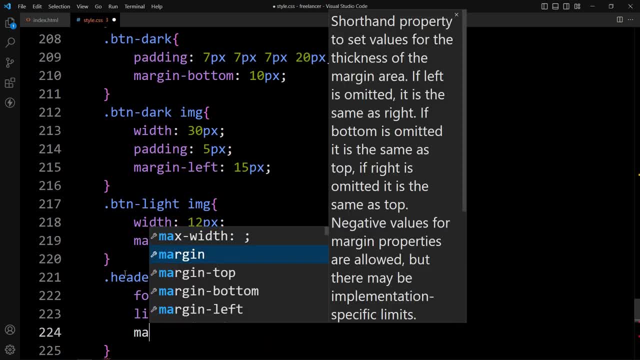 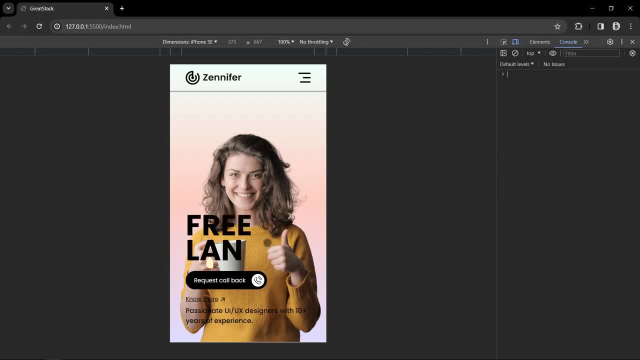 of 60 pixel margin at the bottom, so after adding this, you can see the perfect size for this text. freelancer. now you can see this text is overlapping this image and the paragraph text is also overlapping this image, so sometimes it is difficult to read this text clearly. that's why we will add one. 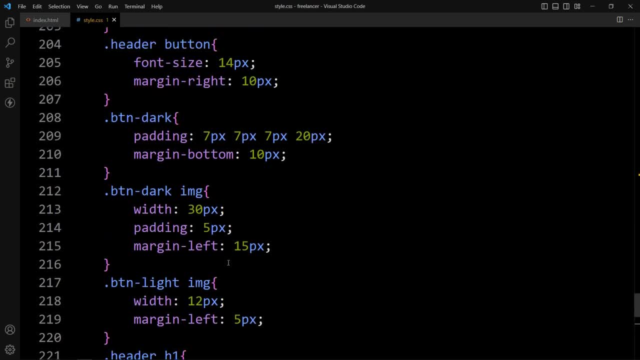 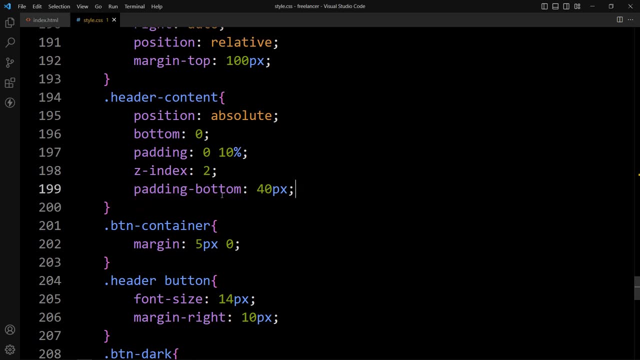 colored layer. so let's come back, and here we have the header content. so in this one we will add the background. so we will add the background linear gradient and just add transparent. from top it will be transparent and at the bottom it will be white. that's it. after adding this again, 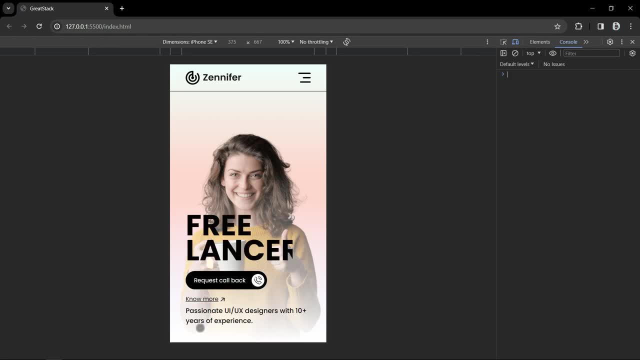 come back to the webpage now. you can see the bottom is white and you can see this paragraph: text is clearly visible. so, finally, we have made this webpage responsive for a smaller screen and it is looking very nice. and let me open this webpage in full screen here also. it is perfect. 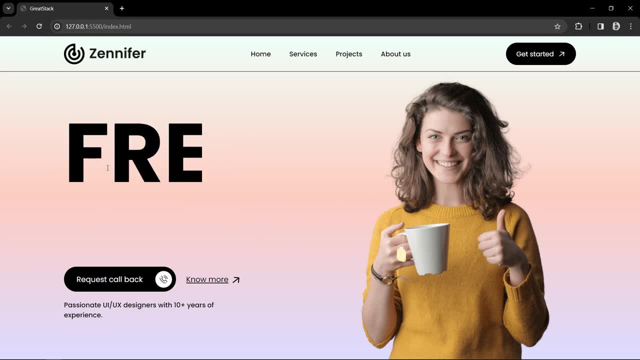 so finally, we have completed this responsive web page design using html, css and very simple javascript. i hope this video will be helpful for you. if you have any question, you can ask me in the comment section. please like and share this video and also subscribe my channel. great. 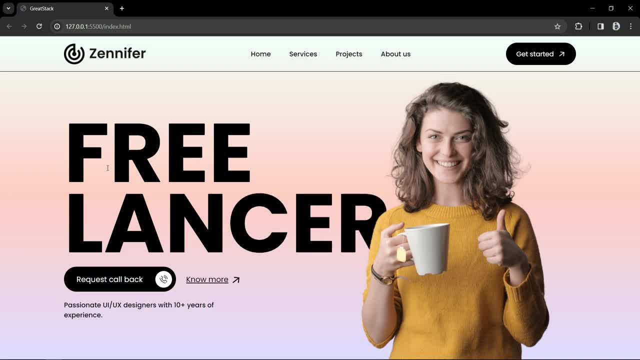 stack to watch more videos like this one. thank you so much for watching this video.